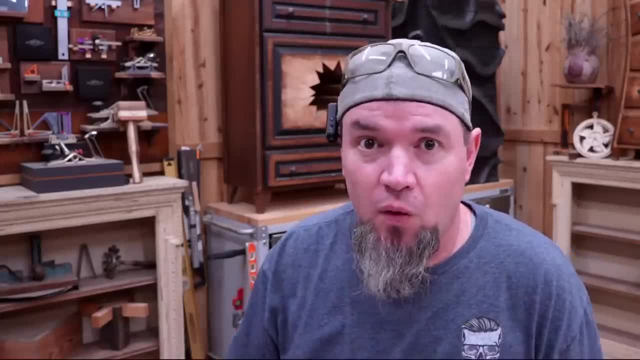 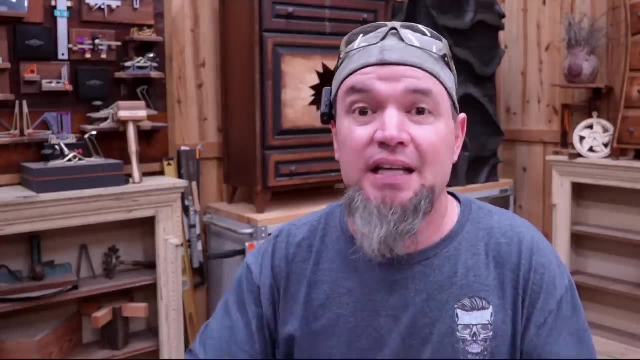 And if it were me, I would actually make both. Like we've talked about before, everyone is different. Everyone's houses are decorated differently, So give people options. And again I cannot say this enough: It is not about what you like, It's about what the customer. 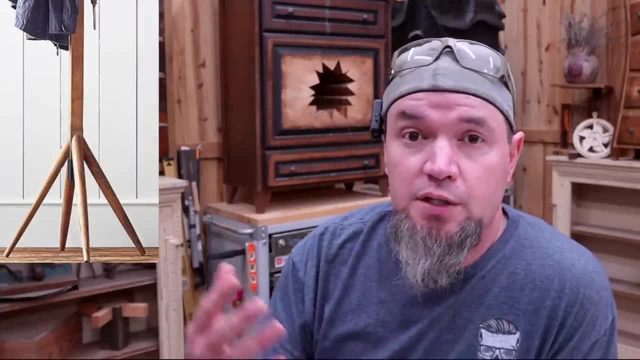 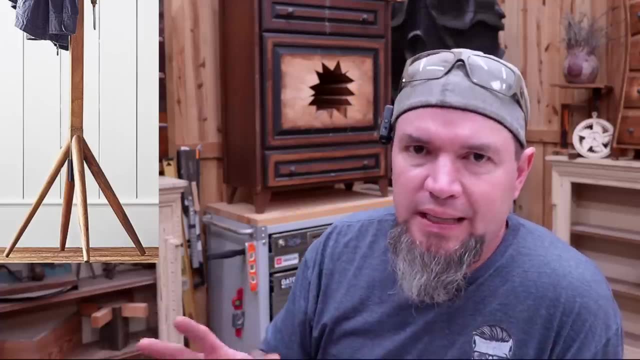 likes. So I'm going to say that you have chosen to use the round legs like this and you've just purchased them off of Amazon. So whenever you get these legs in, they're going to be 16 inches long. That's going to come with some different hardware, but we're not going to be needing that because 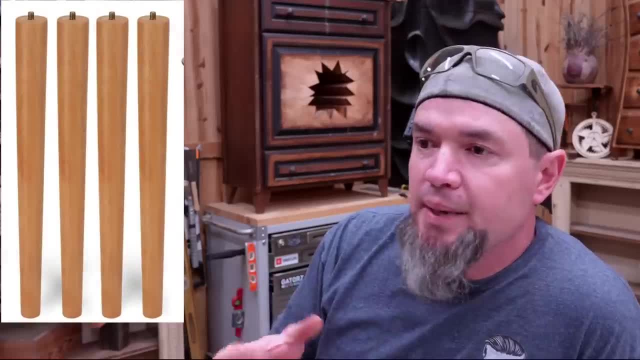 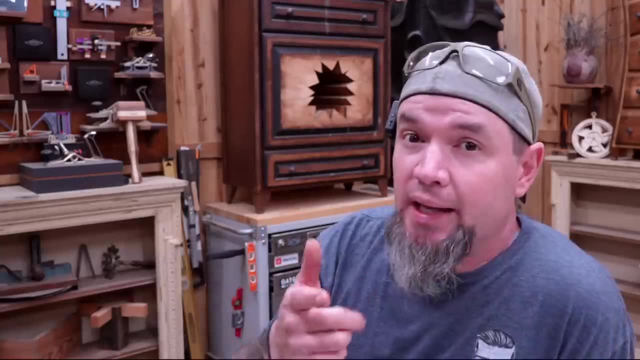 we're going to be needing a sharper angle than what the kit supplies. So when the legs come in, probably going to have a little bump sticking out of the ends. Those are just double threaded bolts. Just take some pliers, unscrew those but hang on to them because you may need them for another project And then you'll. 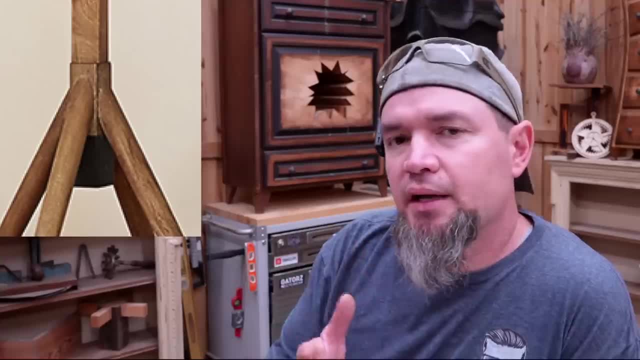 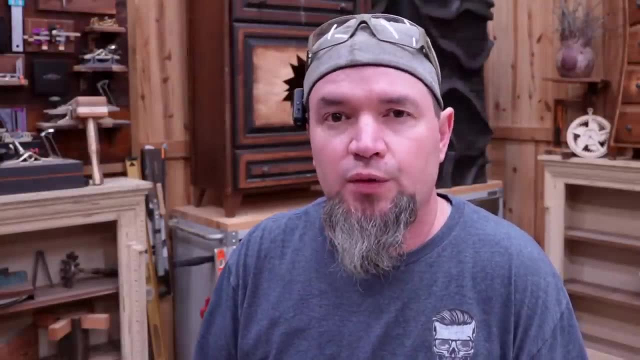 need to put a 50 degree angle on the ends of each one of these. Now, how did I come up with 50 degrees? Well, just kind of playing around. Actually, I just took the span of the base that I wanted, which I wanted right around 22 inches. I took two pieces of scrap, angled them. 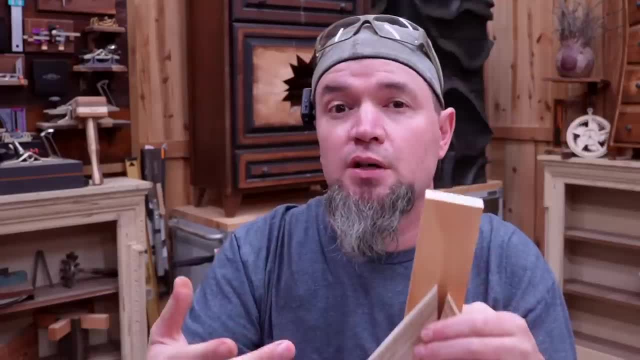 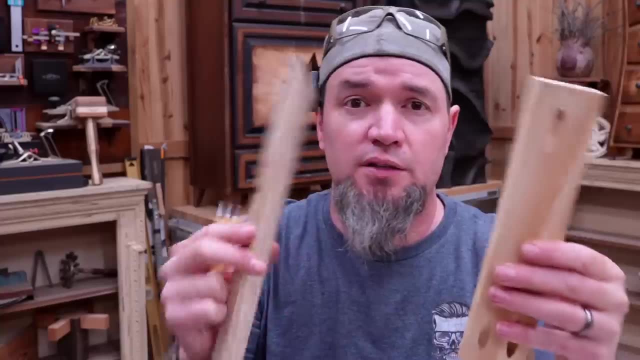 in on a flat surface until they were 22 inches apart. Then just took another piece of scrap that is two inches wide, the same width as our center board, placed it in the center and just marked one of my edges. Took it to the miter, saw, found that edge and it was 50 degrees. 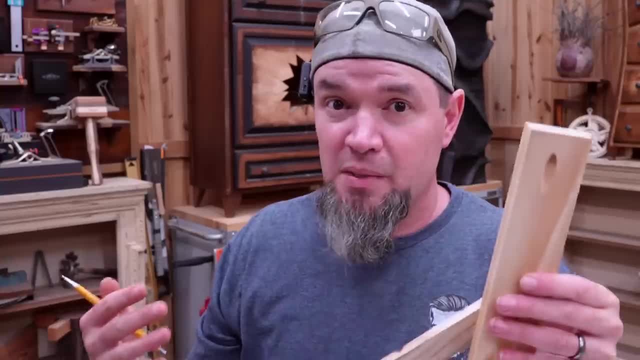 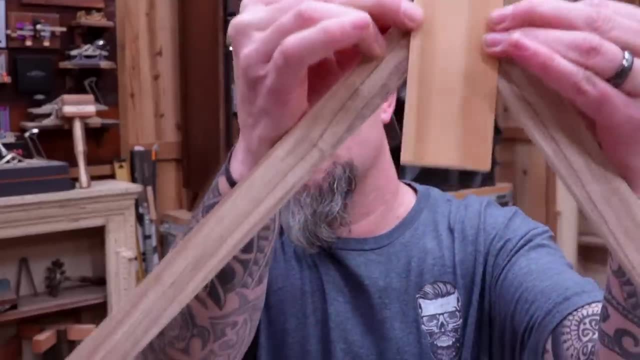 Yes, there are several different tools that you could use to find this, but this only took me about a minute. So, work smarter, not harder. So now that we know that our angle is right around 50 degrees, it's going to look something like this. So, to find the angle, I just use: 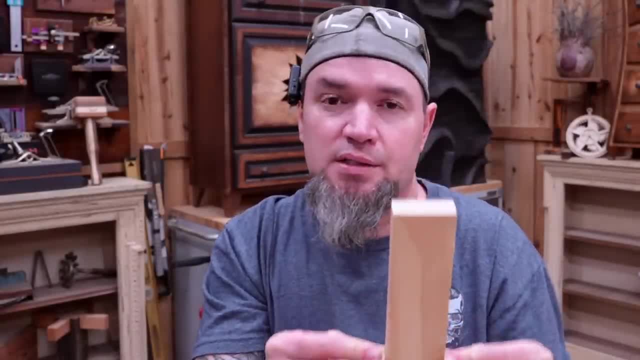 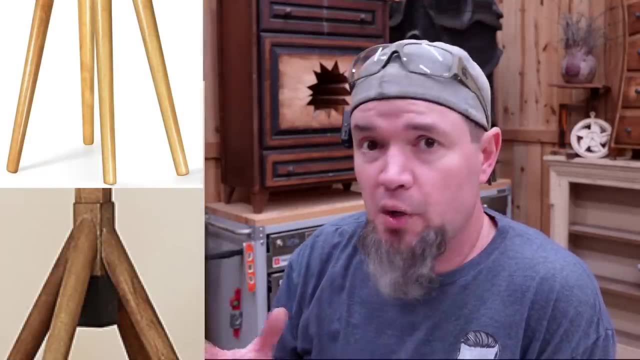 scrap wood and square stock. So if you want to actually make square legs, you just do the same thing. So now that we know that we need a 50 degree angle on each one of these legs, the next step is going to be to cut those. Most people are going to do this with a miter saw. 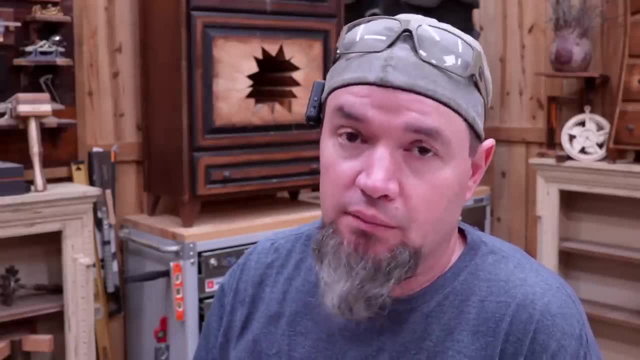 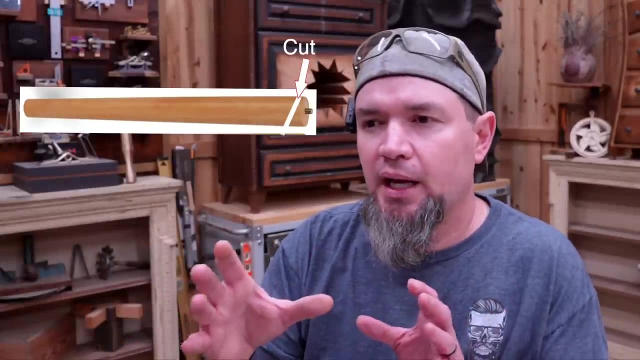 but like anything else, there are several different ways that you can do it. But regardless of how you do it, you have to take into consideration that this is a tapered leg, So whenever you lay this against your fence to make a cut, the back is going to be smaller. 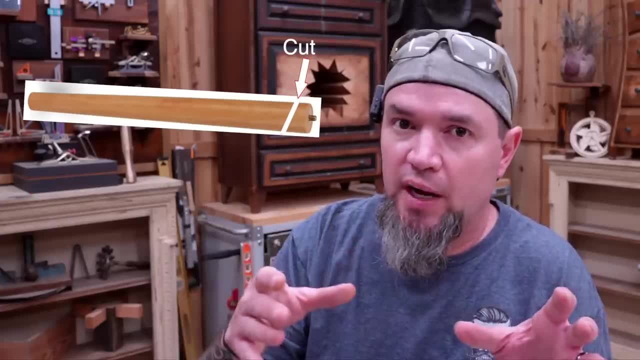 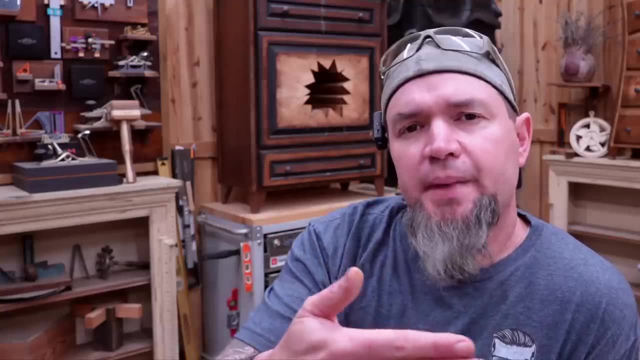 so it will actually shift the piece of wood out of square and changing your angle. So to keep that from happening, that's all that you have to do is measure the width of the thickest part, which is the end that we're going to be cutting, and then shim out the back the same distance away from the 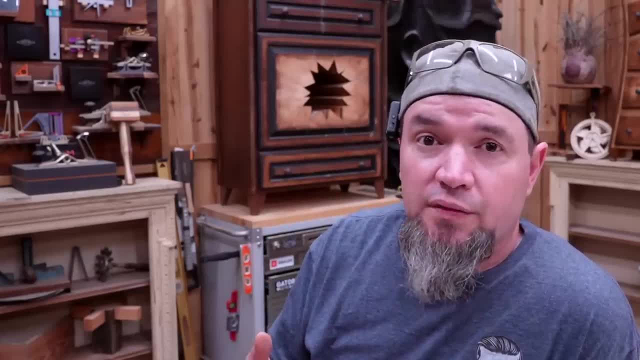 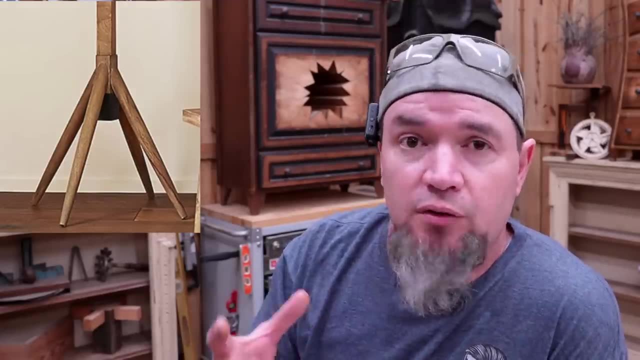 fence. that is the same as the front of your leg. So now, with the leg square against your fence, you're ready to cut your angle. So now, with the angles cut on all of our legs, how are we going to attach these to our 2x2?? Again, there's several different ways that you. 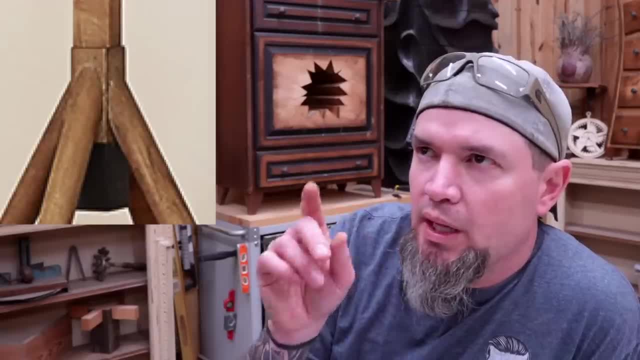 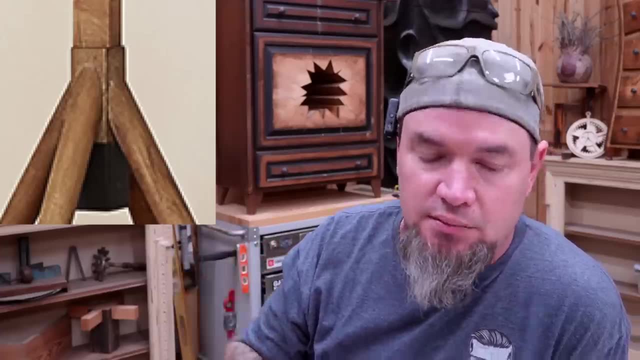 can do this, but I'll tell you how they did it. So if you look close at where the legs attach to the 2x2, it almost looks like that. it's a little thicker at the bottom, like it's designed into the base. Well, it's not. So all that they've done is taken a quarter of an inch piece of plywood. 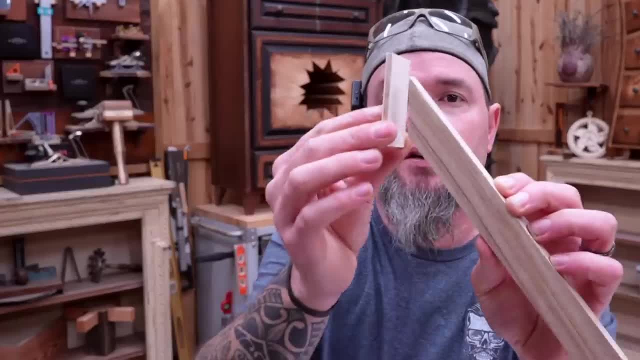 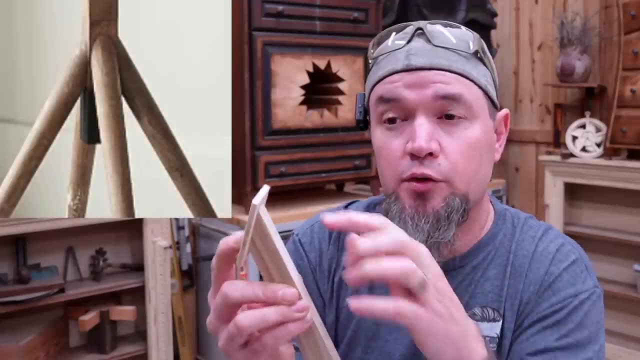 that is the same width as the board- two inches- taken the 50 degree angle and attached it just like this. By doing it this way, it keeps you from having to cut your leg. So now, with the angles cut to install any of your screws or nails at an angle, you can do it all from the back. So I 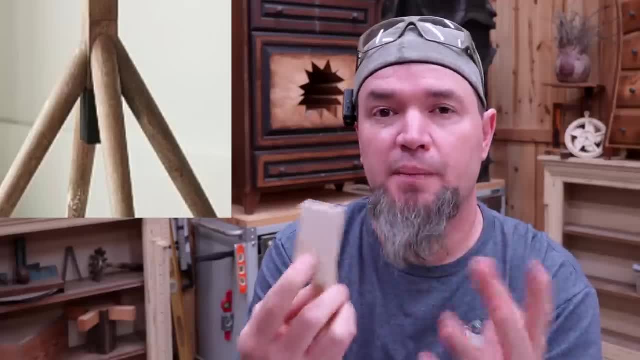 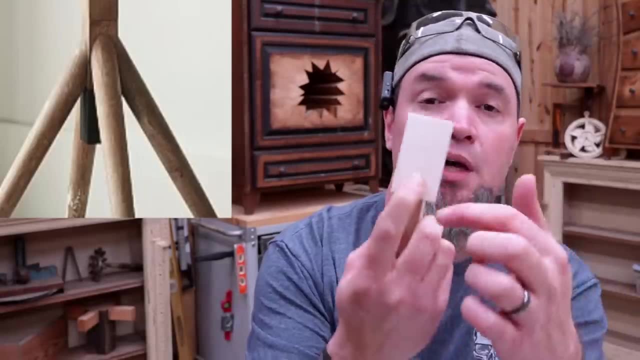 throw on some wood glue pre-drill and put two screws in this. That's going to make for a really solid leg, And this piece of plywood is going to add extra surface for glue. So then, once you have that installed, I would just coat this with glue. measure up maybe four inches from the bottom of. 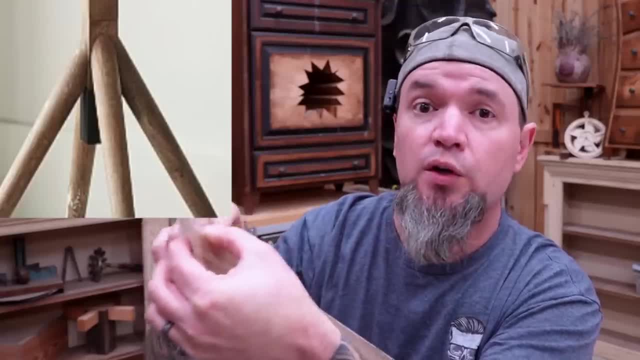 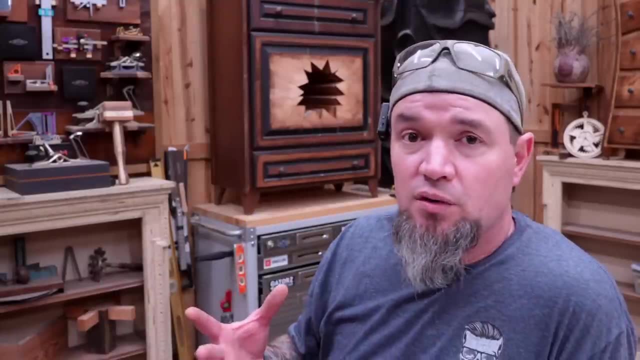 your center board and then attach this to your center board using that wood glue and some brad nails. Once that wood glue dries, you're set, And then you would just repeat this for the other three legs. So, once your legs are on, there's only one thing left to do, So you're going to 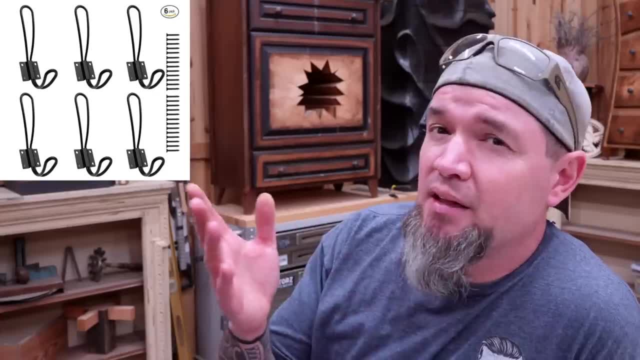 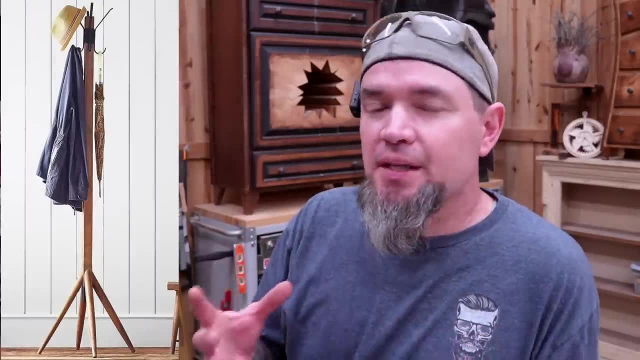 add the hardware. I actually found a six pack of these on Amazon for less than 10 bucks, And once you get one of these on each side of the top, it's going to look pretty similar, And that's how simple that it would be to make one of these Now for me, whenever I would get these legs in. 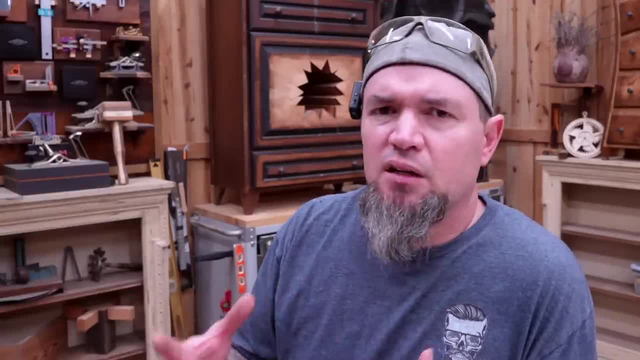 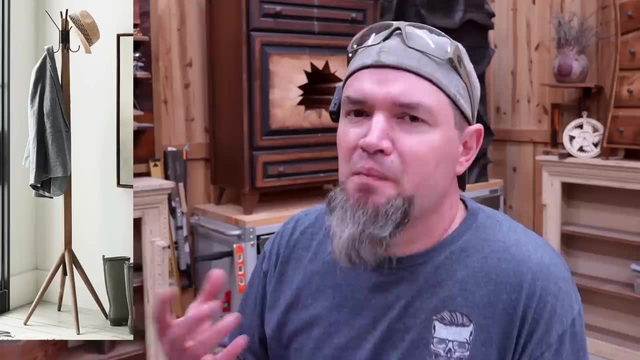 I would sand that finish off, maybe darken it up a little bit and make it look a little more rustic. but to each their own, put your own style and twist to it. And as far as selling these things- 240 bucks is a little steep- You may be able to get that if you're using reclaimed wood. 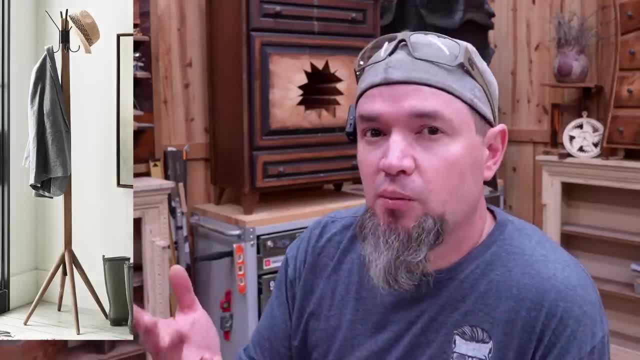 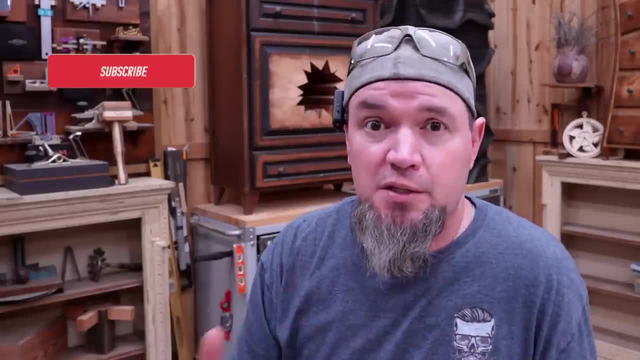 and you're actually turning these legs down. If it were me and I was using new lumber, I'd probably shoot for closer to the $150 range, But again, that's just in my area. Every area is different. We've talked about this before. Things that would sell in my area for $150, you may be able to get. 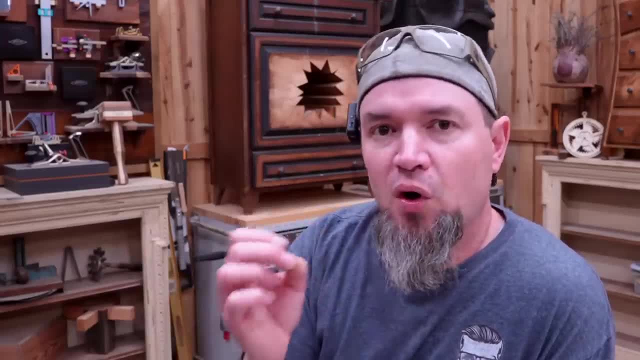 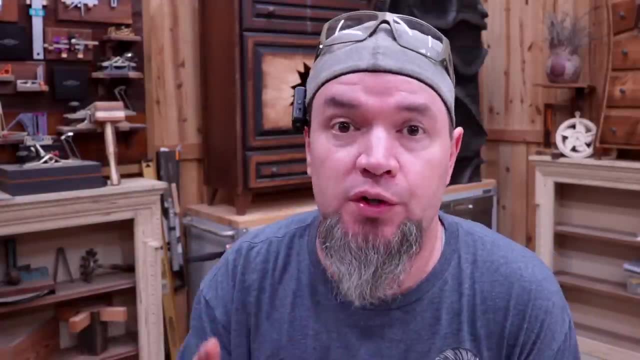 200 out of, And the only way that you can find out is to test the market. This next one I've actually found on tons of different sites, from your fancy furniture places to the actual big box stores. So before I show it to you, the cheapest place and that was a big box store. 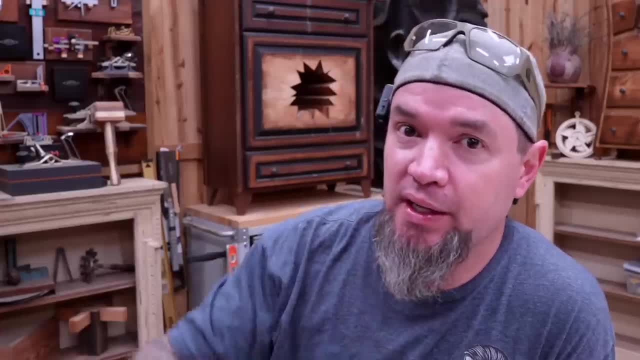 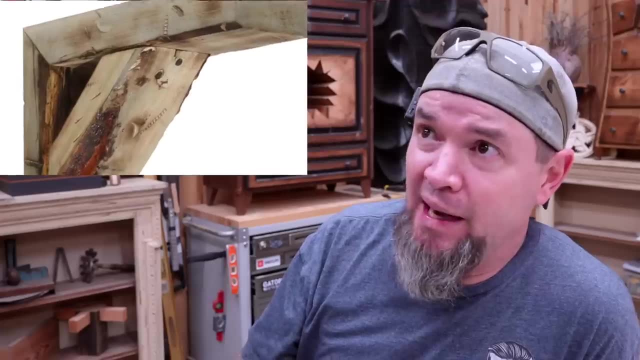 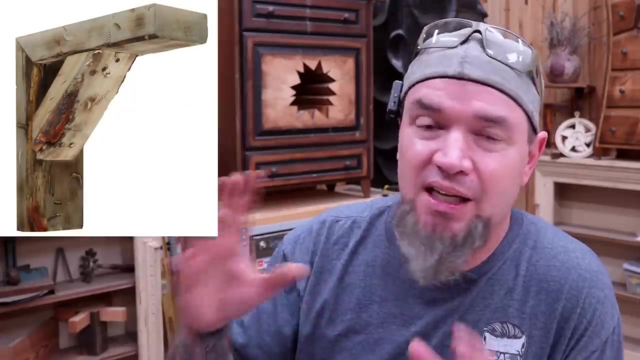 we're selling this for $18 a piece. So they are calling this a vintage farmhouse bracket. I'm calling this a two by four that was made out of a branch that was only about three inches wide. I honestly believe that they are taking the two by fours that they have called did not make the cut And they are making these. 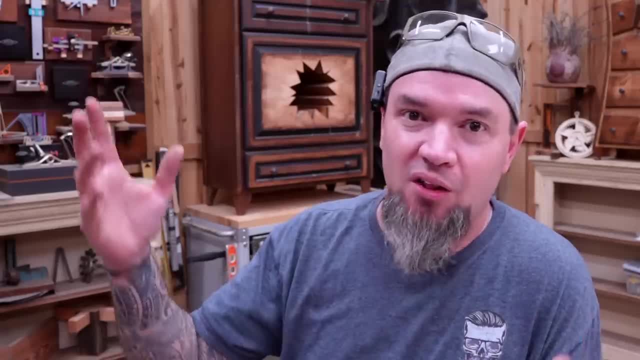 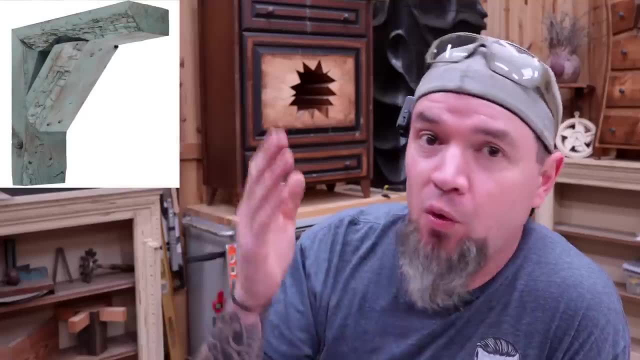 and selling a little piece of that, two by four for $18 to $30.. But anyway, since they were on several different sites, that means that people are buying these and they are popular. You know what to do with this? The board that goes against the wall is 10 inches long. The board that acts 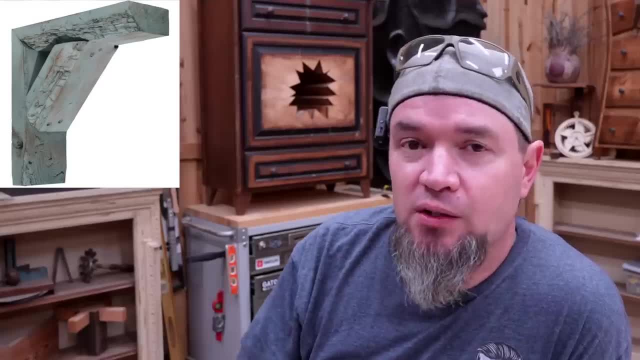 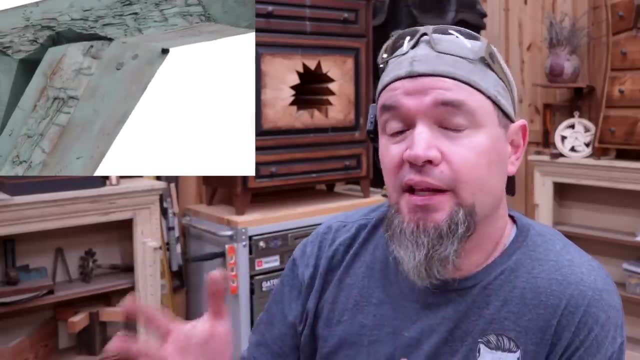 as a bracket is eight inches long. So all they've done is cut 45 degree angles on those two boards, put a couple of screws in from the top, because it's actually going to have a board on top of it, And then for the support bracket in the middle, I'm going to say that it's about six inches long. 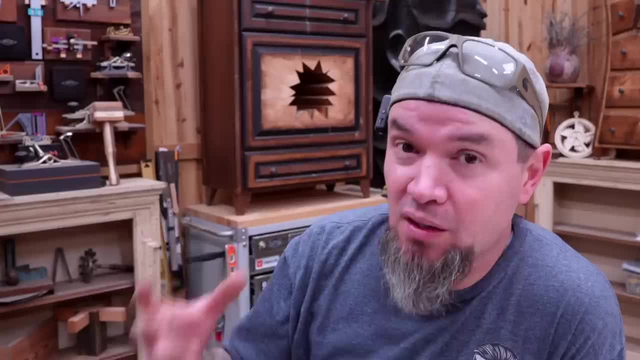 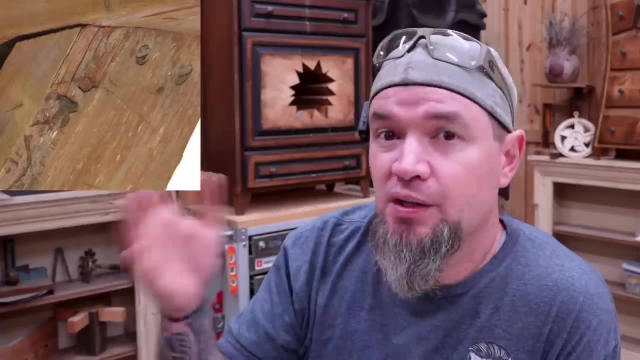 with a 45 degree angle on each side And to make this thing look rustic or look farmhouse, they have taken a framing nailer and toenailed in some nails to hold that into place. You can tell that it's been put in by a nailer, but the nails are actually inset into the wood. 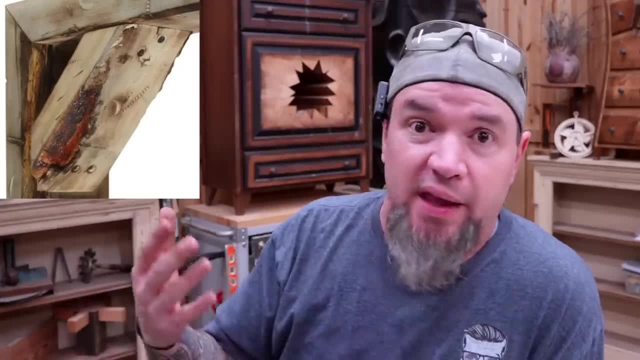 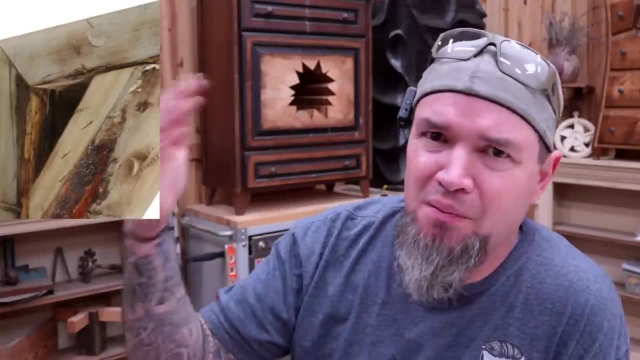 And then that's all that they have done is roughed it up some more Where the bark was showing. they really didn't have to do anything because that's on half the two by fours you find anymore. But then they've taken hatchets and made some marks. You can. 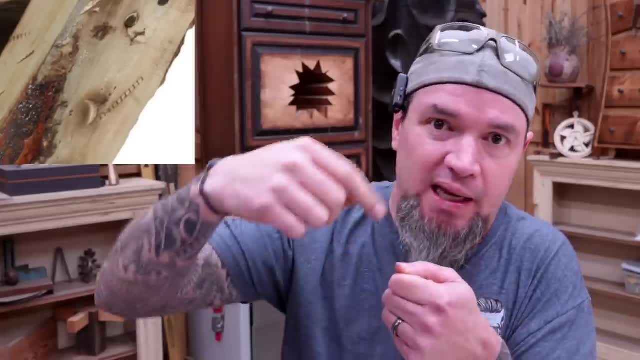 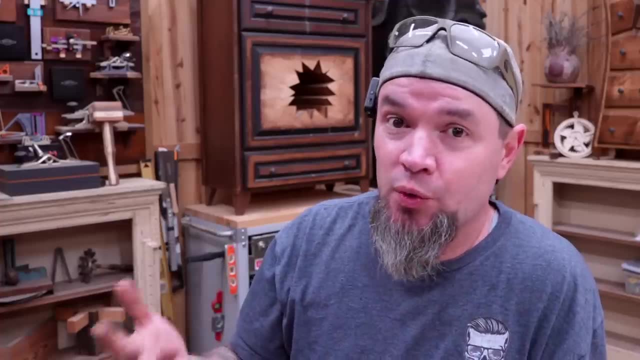 actually see where they've used a screw just to lay onto the board, hammer that in and then put the screw marks in. Why a screw? if they're wanting this to look rustic, I would have used a square nail instead of an actual screw. but to each their own. And then once, all that was crudely. 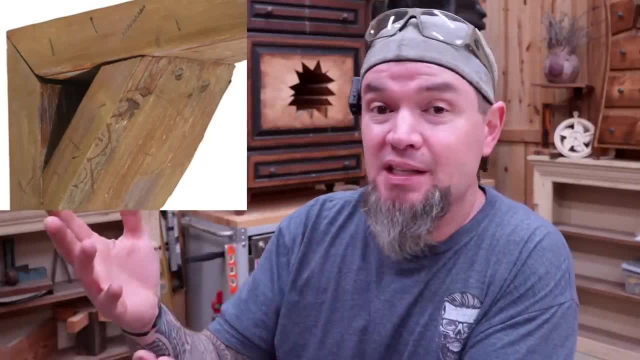 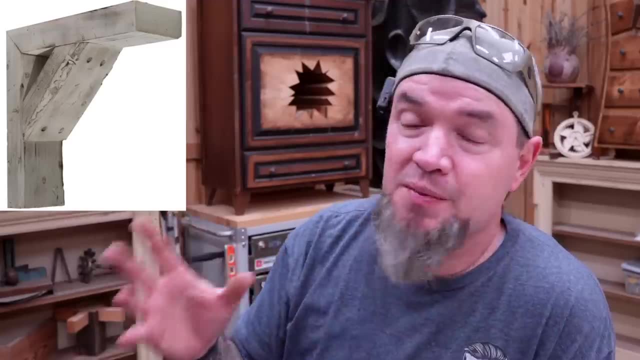 put together, you can see the big gaps. You can see all of that And it really doesn't matter, because that's the theme, That's the look for this. But once that was together, they just slapped some paint on this and all of this paint has been sprayed on. Why they pick some. 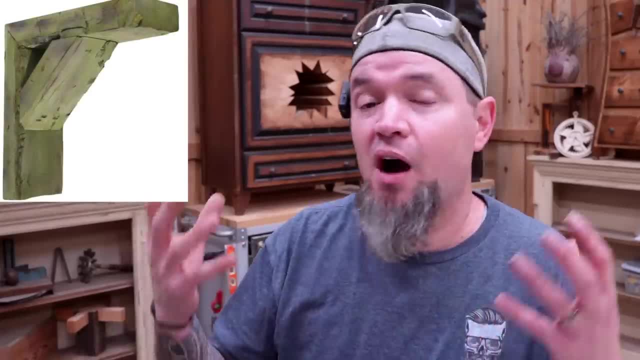 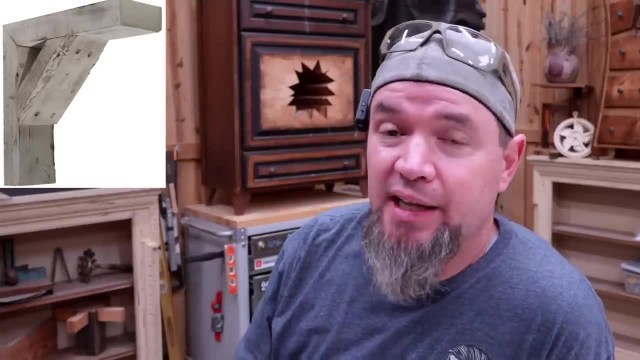 of these colors, like this green one. I have no clue, but they are obviously selling these things. So altogether to build one of these there's only 24 inches of two by four. So that means out of an eight foot stick you can make four of these. So less than a buck a piece. they're selling these. 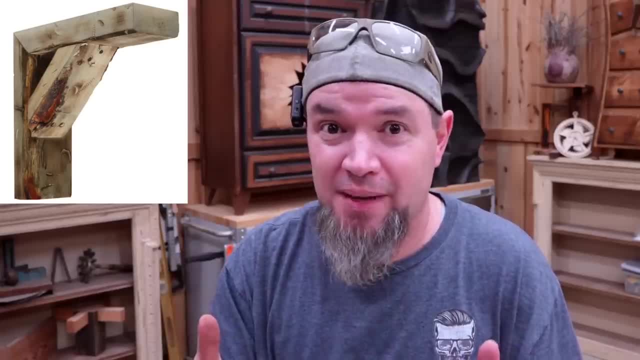 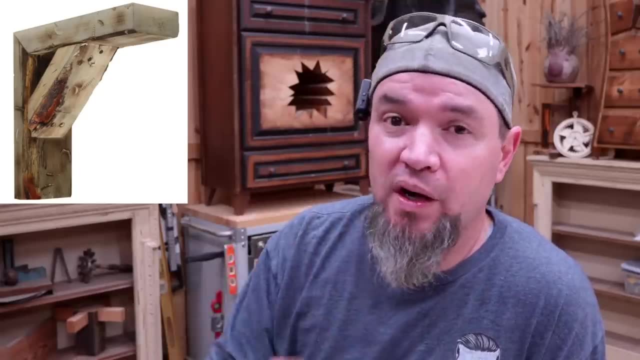 things for 18 to $30.. I'm going to let you decide on what the price these at, because I have no clue. I'd have to test the market and see what people are willing to pay. But the cool thing about this is, if you buy one, you know that they're at least going to buy two And if they're planning on using 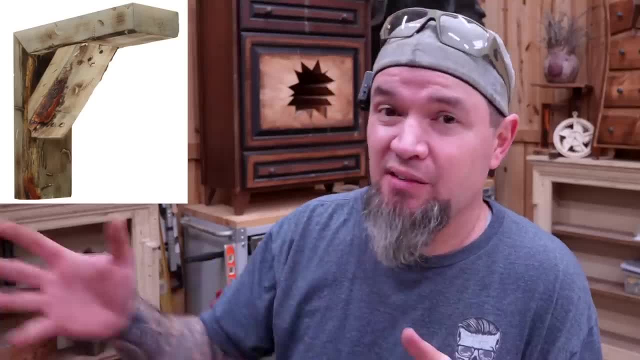 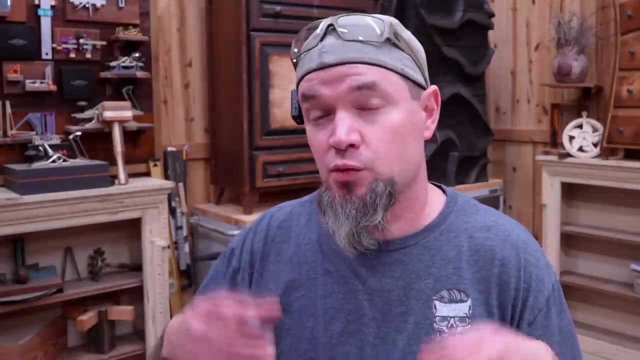 this for a shelf. make sure that you take that scrap piece of two by eight that you have laying over in the corner, because it's all roached out and the edges are gone and painted up to match your brackets. And this next one caught my eye because it was relatively expensive and it was 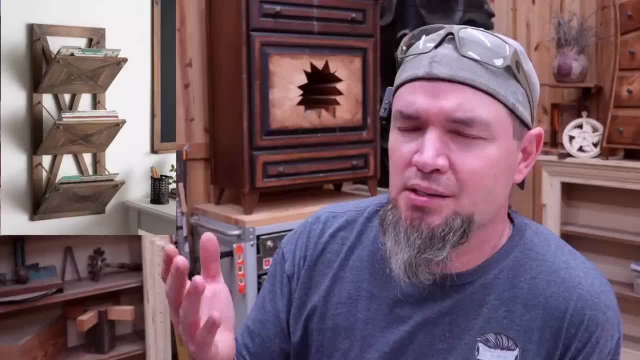 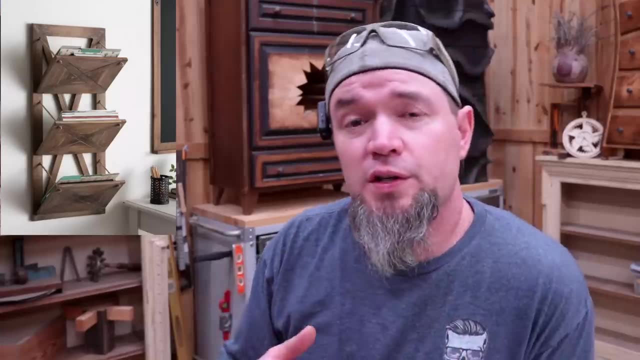 from Target Or when you're trying to sell something like this for a high price, we'll call it Target. Okay, It sounds a little more fancy and obviously fancy name places get higher prices. So regardless of what you want to call the store, this is a pretty cool item and you can. 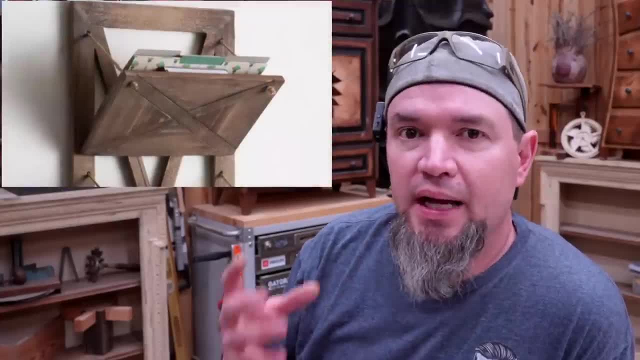 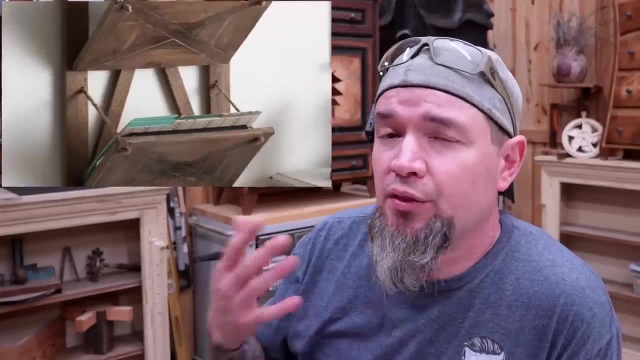 get this out of fence pickets or pallet wood. So they're calling this a three pocket hanging file holder. So when you first look at this build, yes, it may look a little complicated, but it's not If you really take a close look. there's really only three main elements to this. You have your. 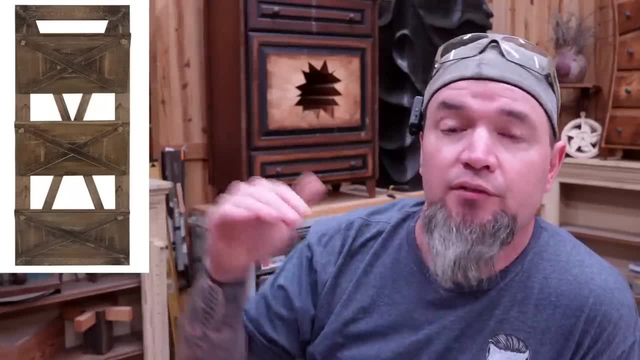 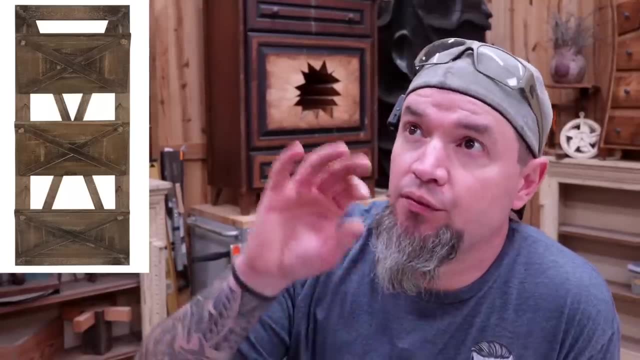 frame that goes around the outside, You have your X brace that's in the center, and then you have your three fold down pockets. So this file holder is 15 inches wide by 33 inches long. So what I would do is start with the frame of this, the backing, And to me it looks like it's all two. 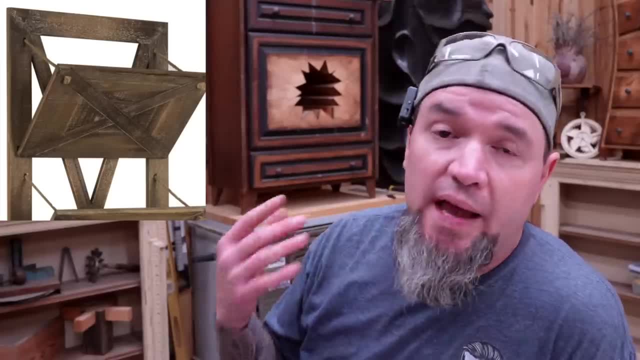 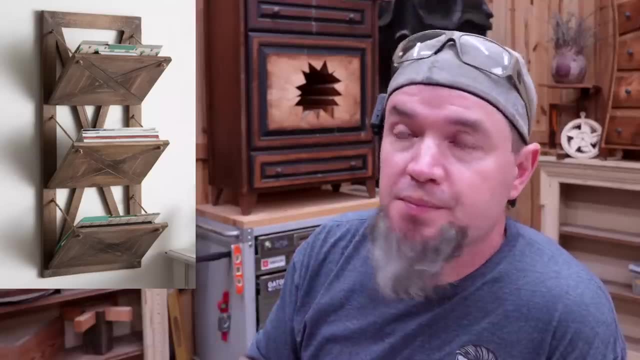 inch material, And then the description of this item. it says that the wood is half of an inch thick, but again perfect for pickets or pallets. So we'll just start by cutting whatever material that you're deciding to use down to two inch strips, and then whatever length and 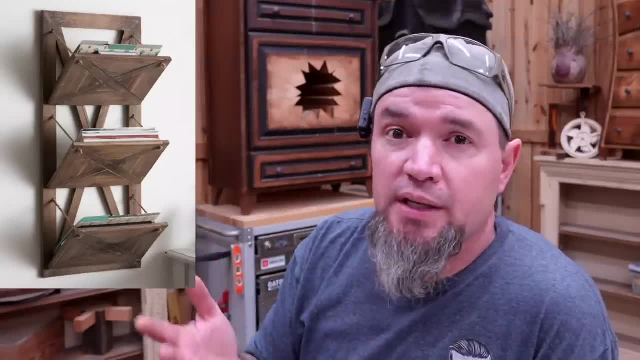 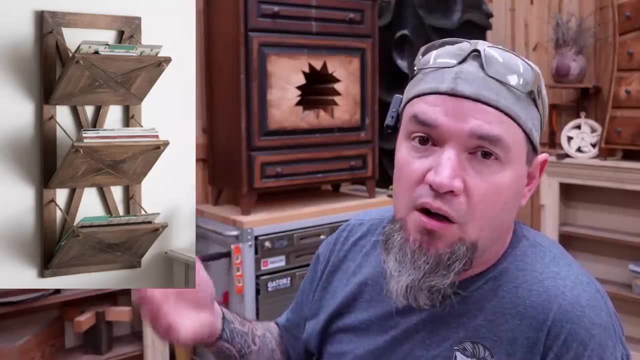 width that you actually decide to build this. Well, let's say that you're going to build it similar to this. So you need two outside boards that are 33 inches long, with 45 degree angles on each side, and then the top and bottom board 15 inches long again, with 45s on each end, And then 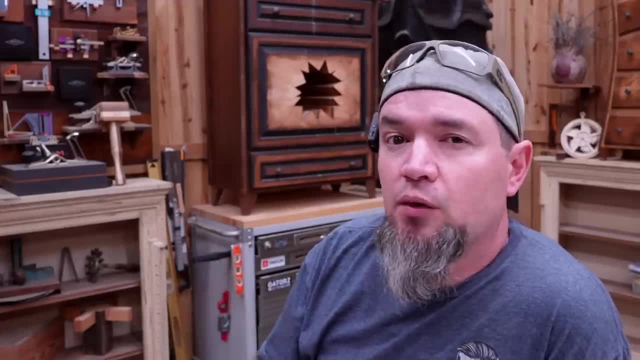 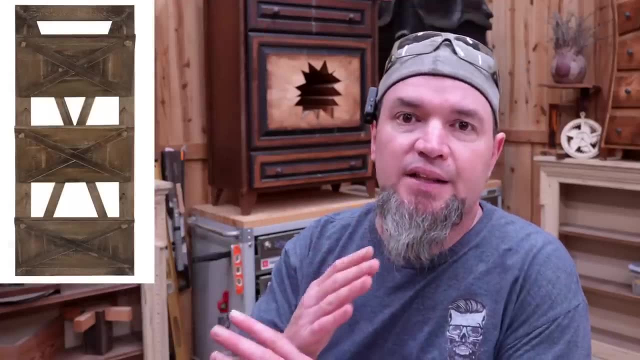 we'll just put this together like we would a picture frame And then for me I'd put it together with some pocket hole screws in the back. Super fast, super easy. So once you have the exterior frame built, we'll move on to this X design in the center. If you look at the corners of this thing, 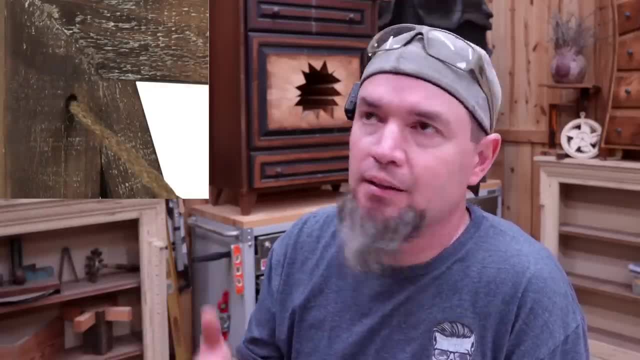 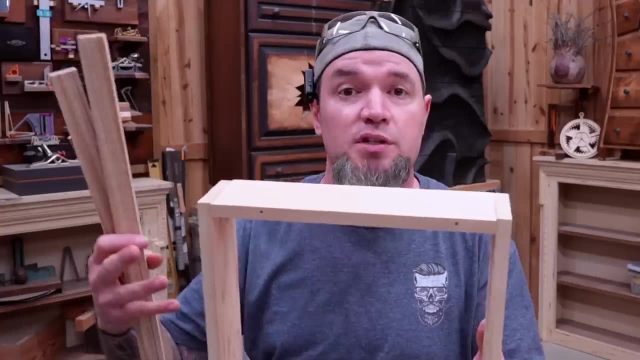 it looks like that there would be all kinds of complicated angles and things like that. Let me show you a super easy way to mark all of those cuts without using any type of math or angle finders. We're going to say that this is a rectangle, for whatever size that you decided. 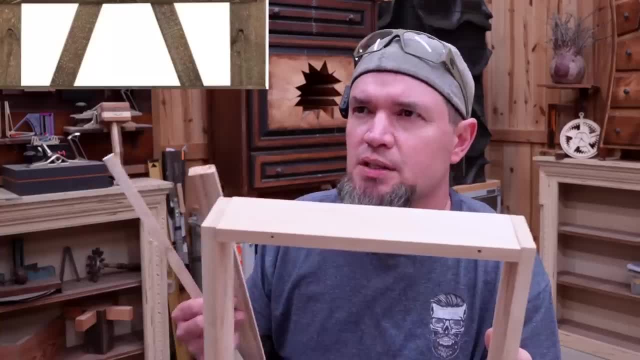 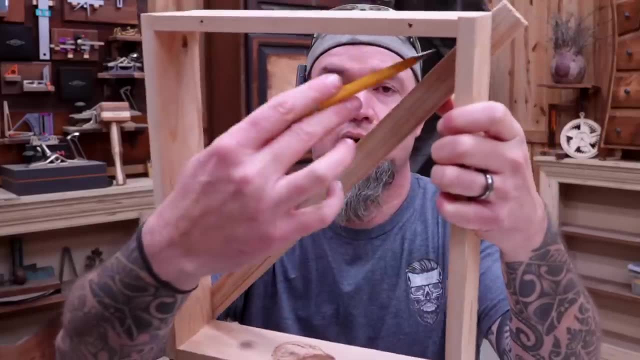 to build the outside frame, You would take two half inch strips, and theirs looks like that. they're about an inch and a half wide, but go ahead and cut those a little long. And then what I would do while the ends are square, I would lay my first one across from angle to angle. 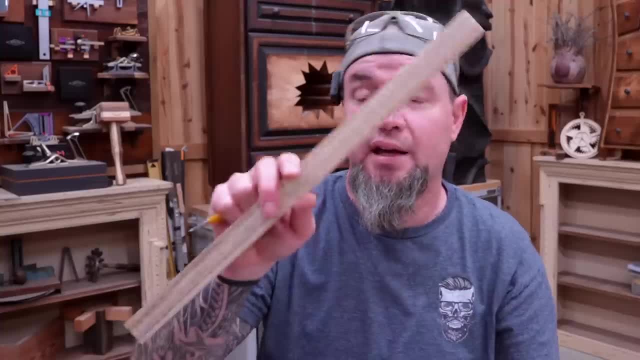 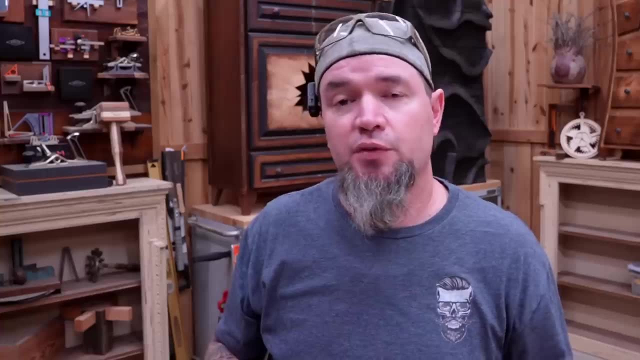 and then, from the inside, make my mark on both sides- Now that I have my two ends marked, head over to the miter saw and make those cuts. Now, if you've made this thing perfectly square, you can make those exact same cuts for. 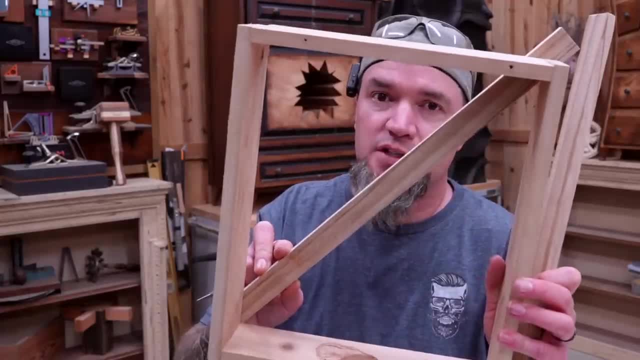 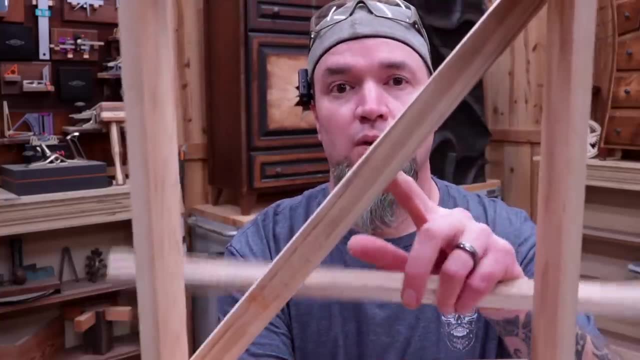 your second board. If you're a little worried about it, just do the exact same thing for your second one. So once you have your outside angles cut, you could either put a half lap on both pieces in the center or you can install your first full length piece, lay your second one. 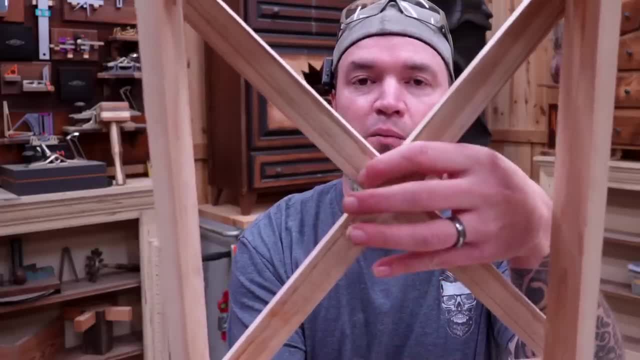 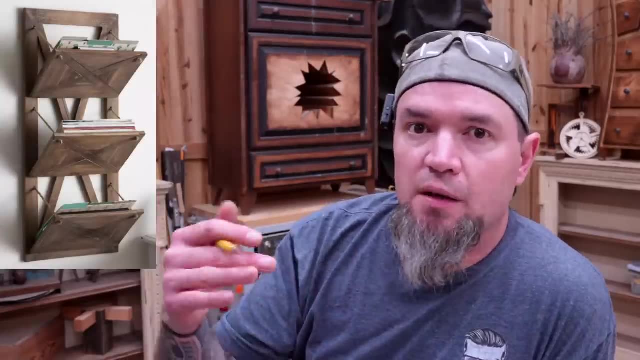 on top to where it fits, and then draw a line on the top and the bottom. Then you can make those two cuts and then everything would fit in flush, giving you that design. So now you have the entire back done. So now let's talk about the hanging folder shelves. 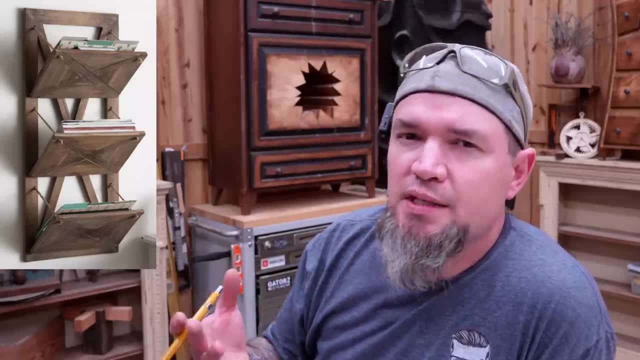 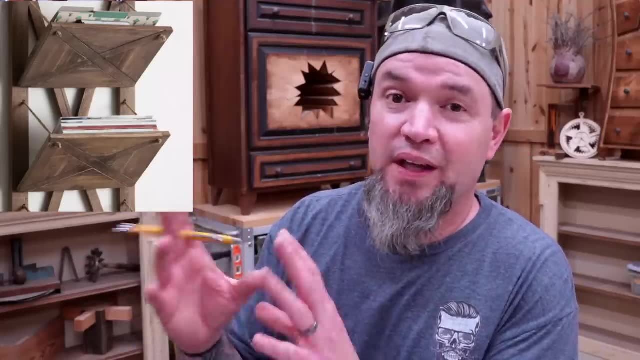 I'm going to estimate that, if this is 15 by 33, that each one of these panels that they're using are probably about 10 by 15 inches wide. So these panels are a lot easier to make up than what they look. So it looks like that they've made it like a cabinet front where you have your four outside. 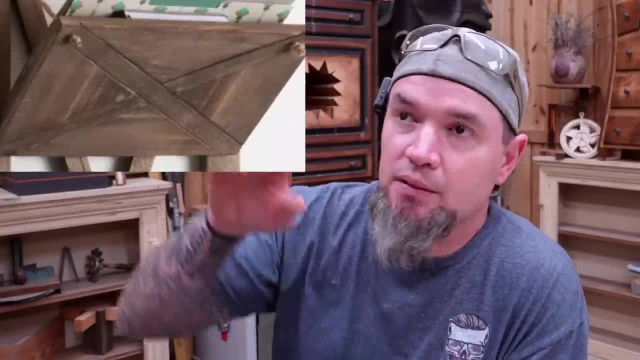 pieces and then you have your inset board in the back. but that's not the case If you look really closely, not counting the X design in the center, but everything else is one panel. The only thing that they have done is darken. 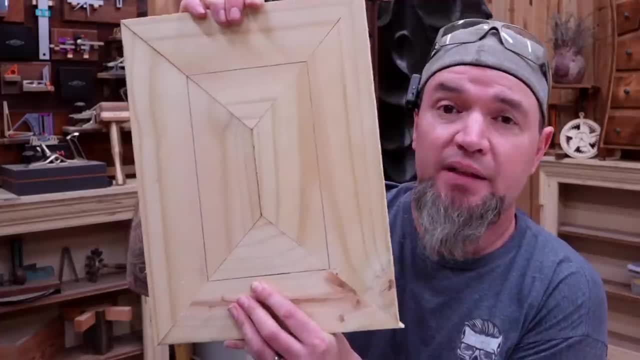 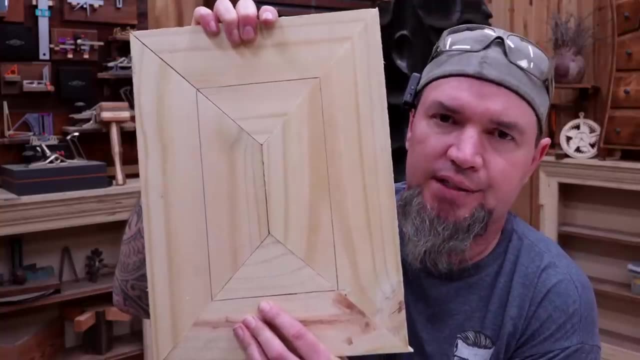 Center to make it look like it's recessed. Let me show you what I mean. So I just made this out of some scrap fence picket ends that I had laying around and it's a 15 by 33.. And obviously I haven't done any distressing or anything like that. But if you take a close look at this, 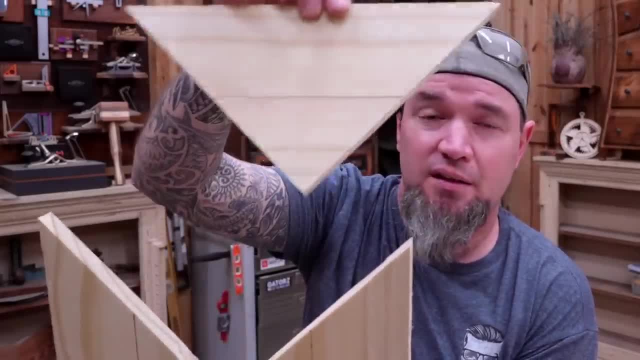 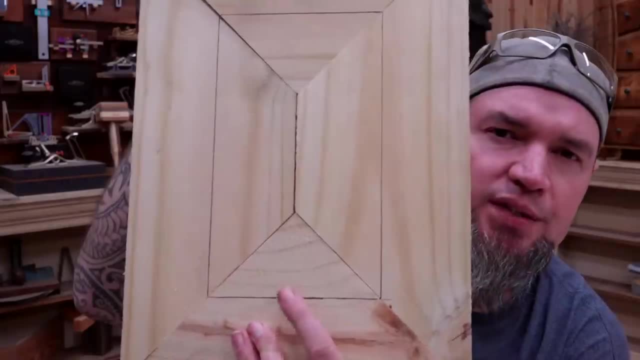 the width is two fence pickets wide And for the ends, the 45 is just meet in the center. giving you this: Okay, So there's your panel, Okay, And you see this dark line that's going around. That's where I would actually darken the center to give it the illusion of depth. 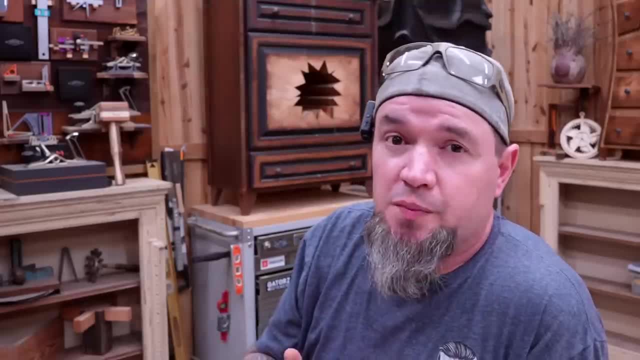 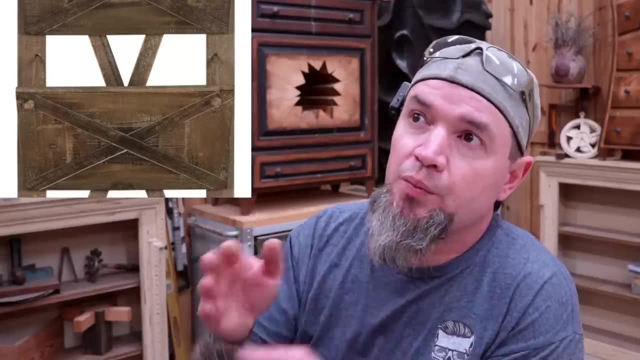 Which is what they've done here. So again, I would just attach all of those parts using wood glue and brad nails. You can use dowels or put some pocket hole screws in the back, But once your panels are made up and you want to put this X design into the center, this is how I would do. 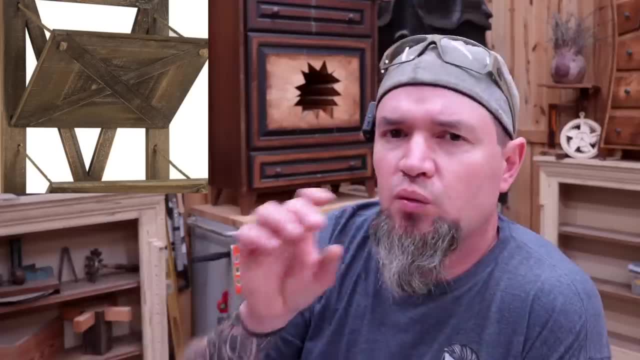 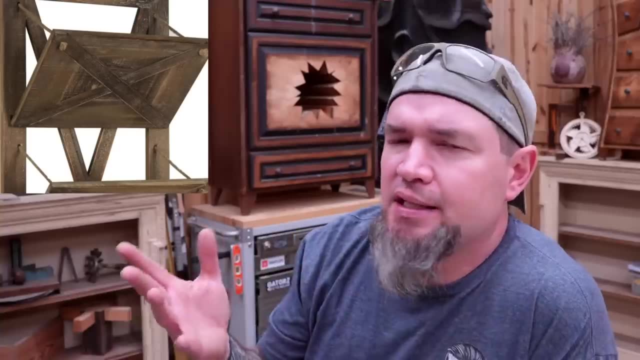 it. I would not inset this design at all. Yes, you could route out those two channels and inset boards into that, or why not just cut some quarter of an inch strips and put them on top? It's not like this panel is inset into anything. So again, you do you, But for me I would just put these things. 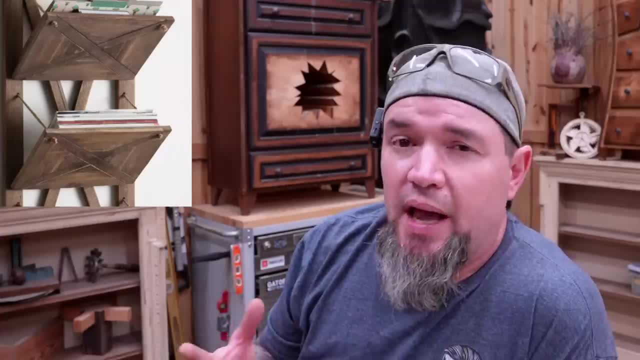 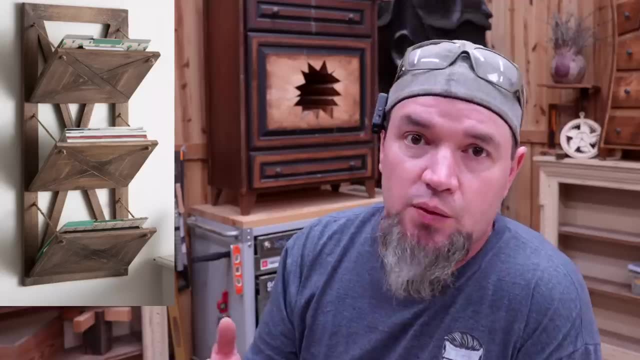 and maybe even skirt the outsides of it with some really thin trim, So you'd actually be adding more dimension to this. Any way that you decide to do it, you get your three panels made. You just lay these out with a spacing that you would like onto your backing And the base of each one of these. 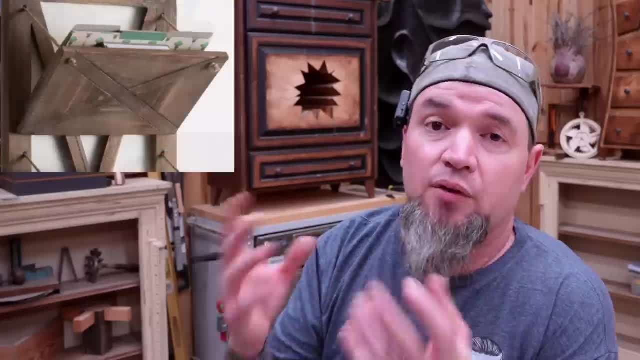 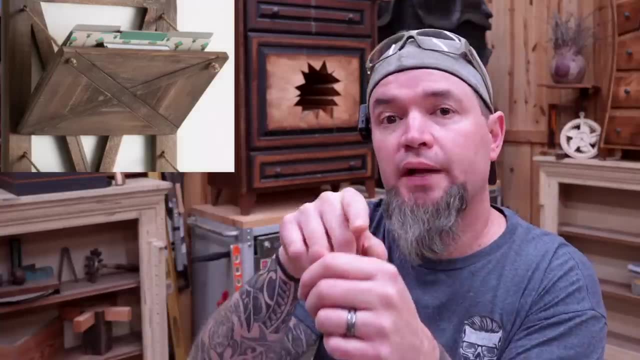 panels. I'm sure that they've just used some really cheap square hinges on each side And for the top to get that angle. all they've done is drilled holes in each end of the panel, folded that panel up and, wherever those holes fell, drilled a hole into the backing And then. 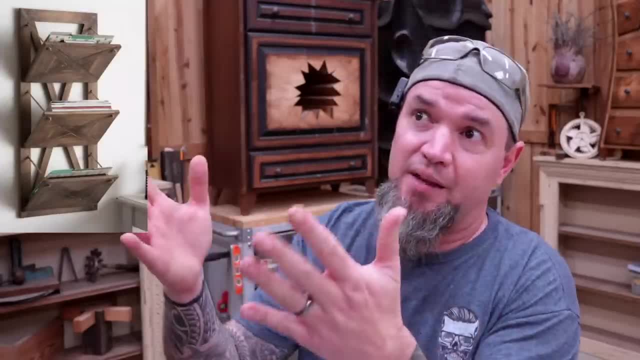 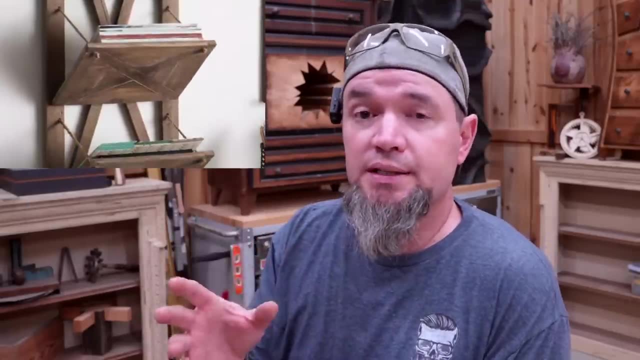 took a couple of pieces of rope, ran it through there, tied knots on the end and bam, you have a three pocket file holder. They're wanting $65 for this, And I'm positive that they have shipped this in from overseas, So for me, I would actually keep the price right around that and focus on the. 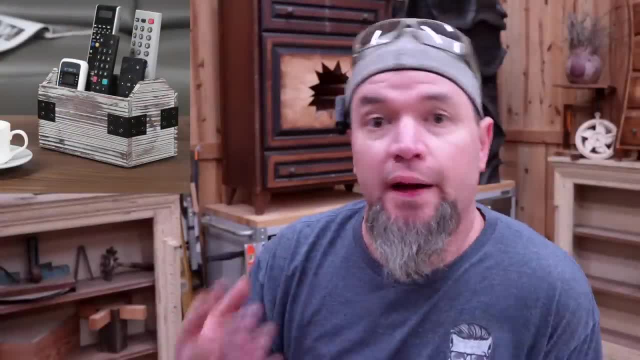 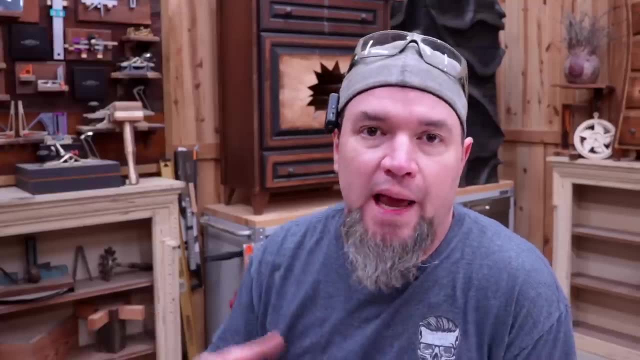 fact that it was handmade by you. And this next one: they are calling this a wooden desk organizer with a bunch of remotes in it, And they're wanting $30 for this thing. Remote caddies and things like that have been around for years And now, of all times, we have remotes for everything, So we need. something like this, And the super cool thing about this one is you can build it dirt cheap. This will make a great fence picket build, because the dimensions on this are four and a half by five and a half by seven and a half inches long, Since most fence pickets are five. 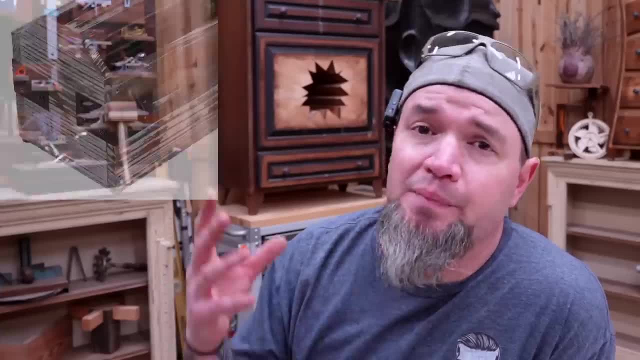 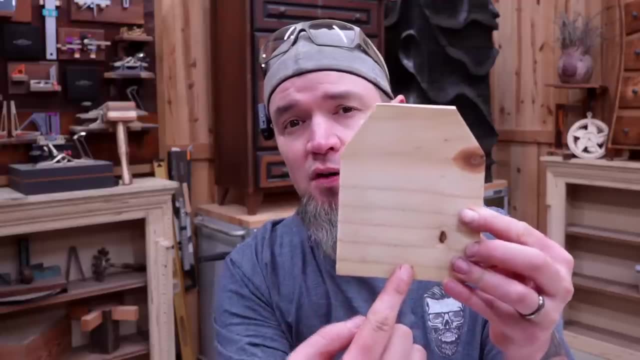 and a half inches wide, Perfect. So let's break this down. The two end pieces are going to be our most complicated part of this whole build, And it's not complicated. This is it. It's five and a half inches tall. Then I cut it at four and a half inches wide. As far as these angles. 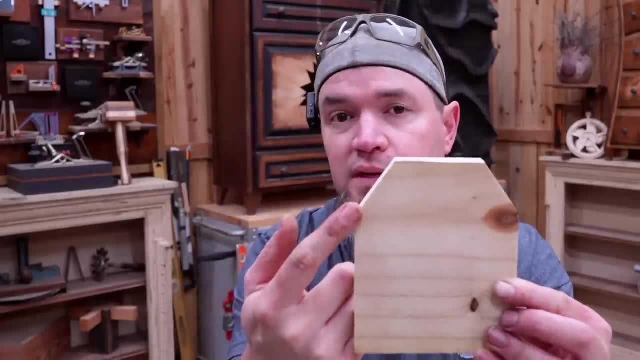 I measured in an inch on each side and made a mark, And then for the bottom part of this angle I measured up four inches Because based on this picture, that's kind of what I figured the sides were. So I had my four. 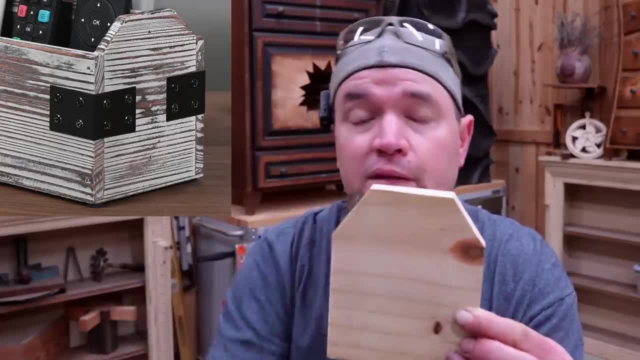 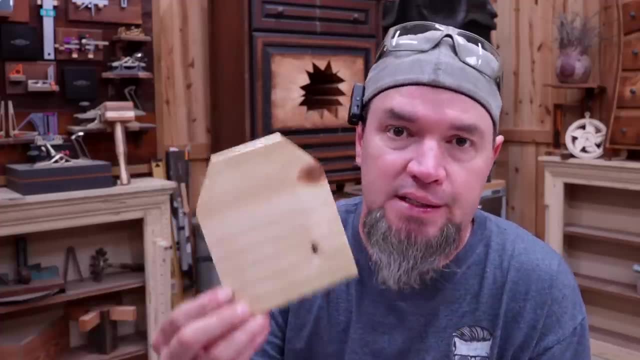 inch mark and then my one inch in. Then I just cut that angle and repeated it for this side. Now I have a template. I can actually lay this on a picket all the way down the thing, if I wanted to, and cut several of these. So we need two of these end boards, And then for the sides we'll need two. 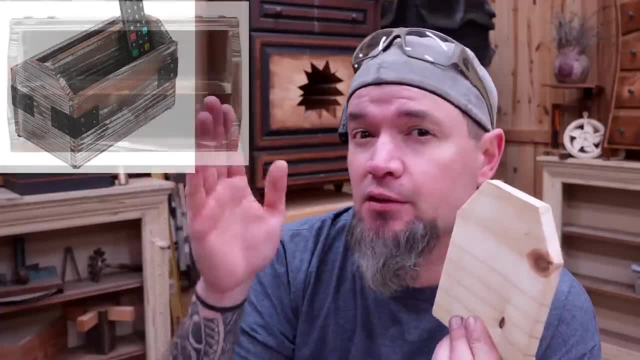 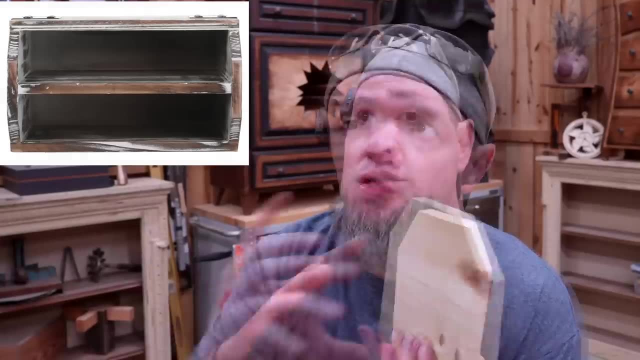 boards that are four inches by six and a half inches long, And then the center divider. we'll need one more board that is five and a half inches by six and a half inches long. For me, I would assemble this with brad nails and wood glue, Starting with the sides. 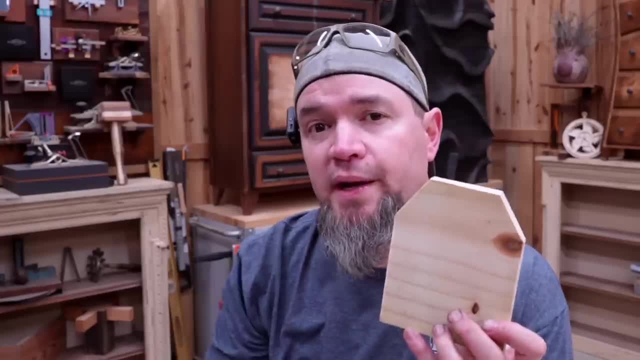 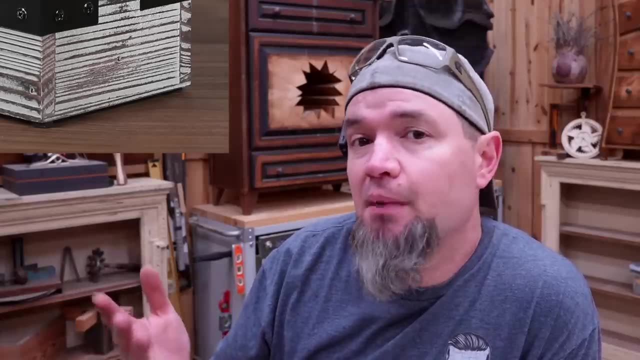 and then slide the center divider down into the middle And then throw in a couple more brad nails from each end As far as the bottom that's. all they've used is a quarter of an inch piece of plywood and tack that from underneath. Now you could inset that bottom if you would like. 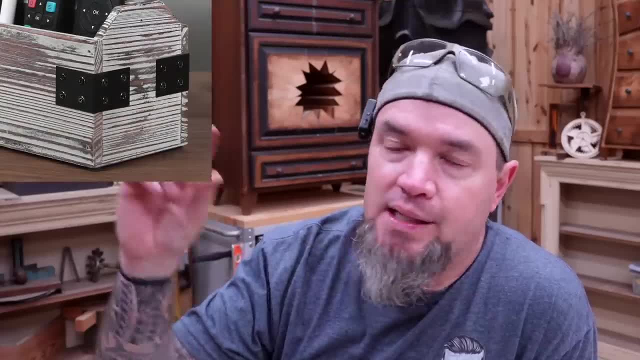 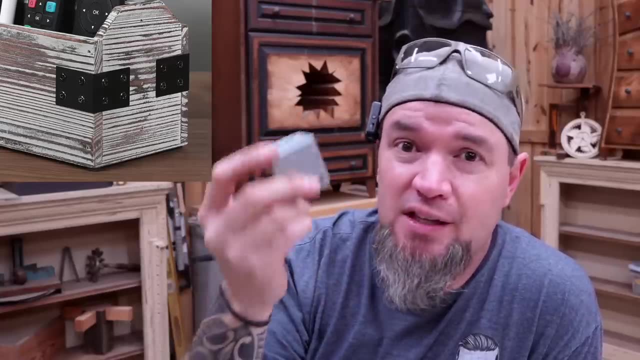 but I really don't think it's needed Now these black decorative brackets that they have going around the sides. This is all they are. So you can go to any big box store, You can go to the lumber and framing section, And these corner brackets are less than a buck a piece. They. 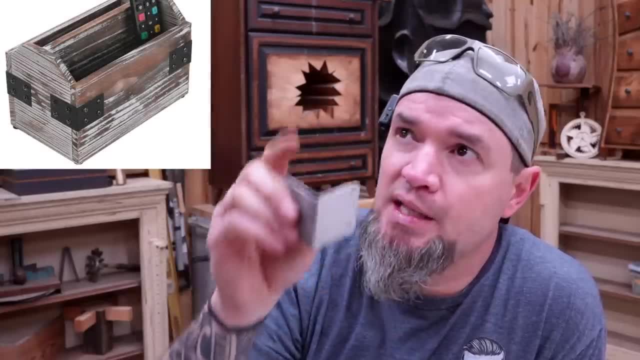 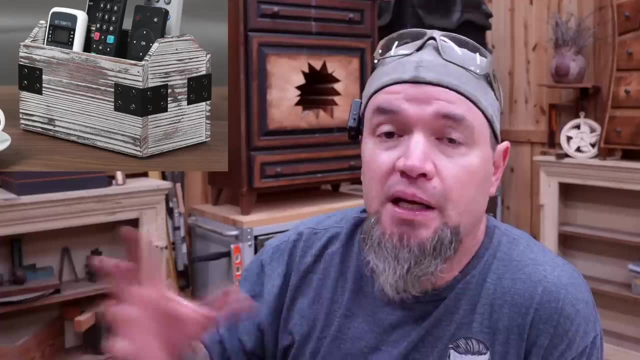 have all different kinds, all different sizes. This one only has two holes on each side. Looks like they have those two. Spray paint those things black And before you install those, go ahead and paint these things up any way that you would like. They've just whitewashed theirs. 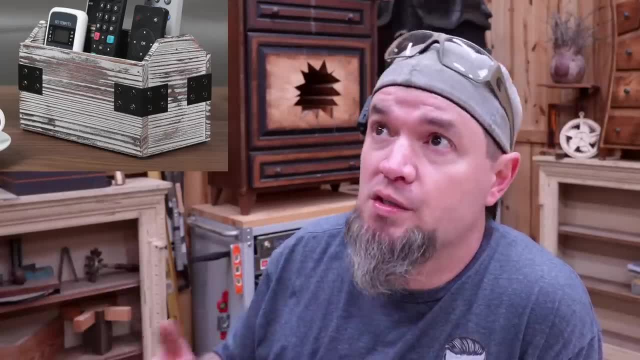 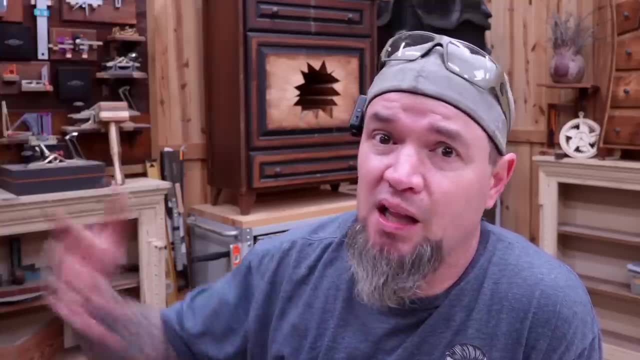 which looks pretty good, and threw the brackets on. If you had all of your parts and your boards were already painted, I'd say that you could put one of these together in less than five minutes. throw a $25 price tag on these babies and let them roll. So while I was looking around, 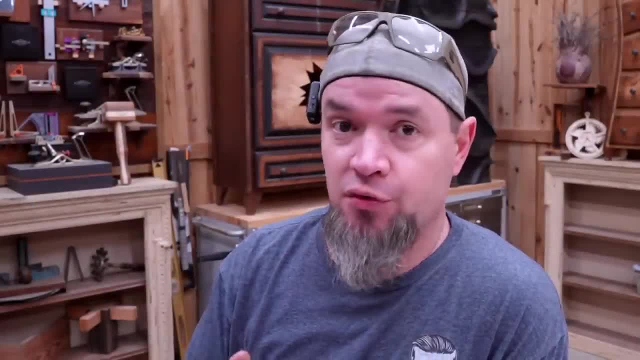 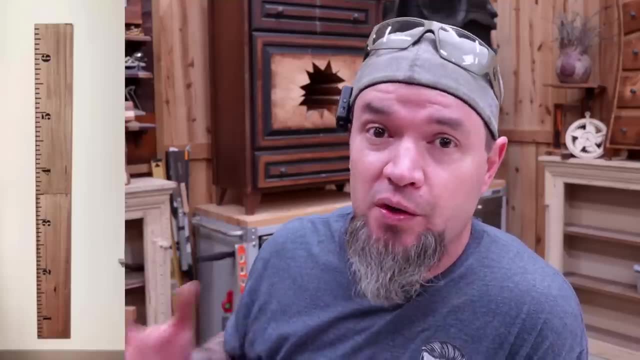 the Tarzay website. and for you non-fancy people, that is French for Target. While I was looking around the Target website because I'm not fancy- I found this And I thought, well, I'm not going to buy this, And I thought that it was super cool. So the measuring rulers for kids have been around. 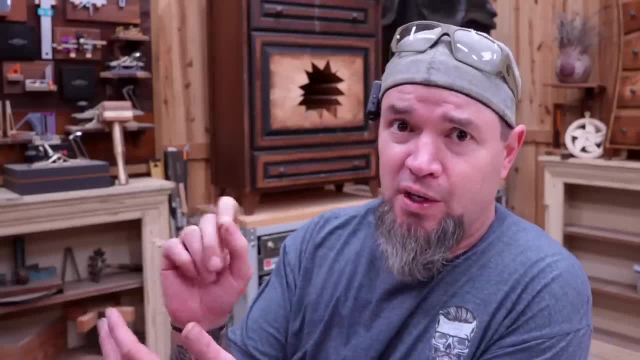 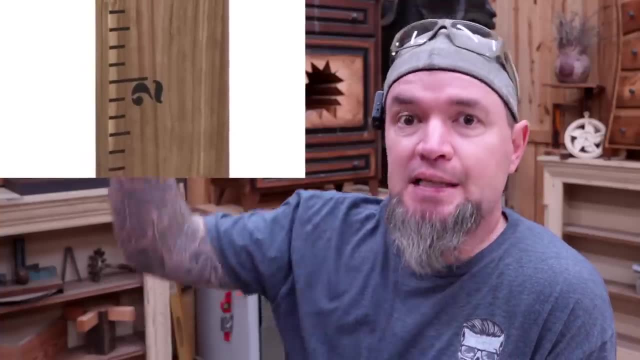 for a long time, I guess, whenever it was no longer acceptable, just to you know, mark it on the doorframe, like we always did. But what caught my eye about this one was it was folded in half. Usually you just see them like as a sticker or something like that. 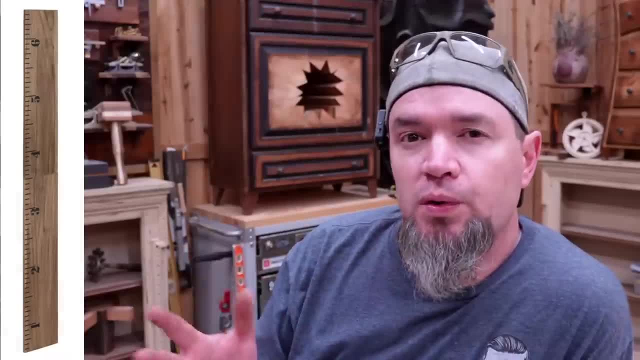 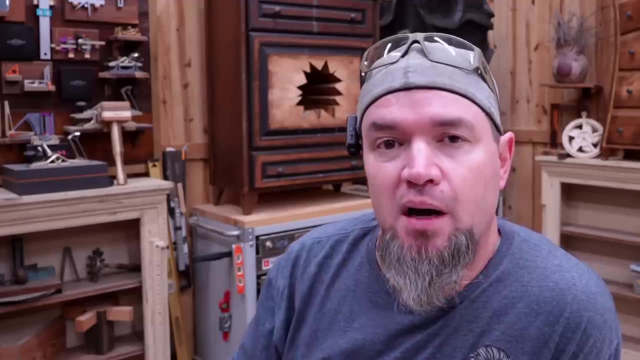 just on the wall, But this was a nice piece of wood that folded up. So this wall ruler is seven and a half inches wide, by six foot tall, by three quarters of an inch thick. All right, so how about a 1x8?? Right now at the big box stores, 1x8s are selling for $10.60.. Let's say that you wanted to. 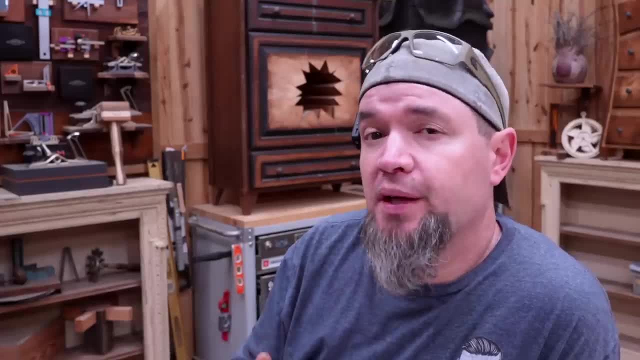 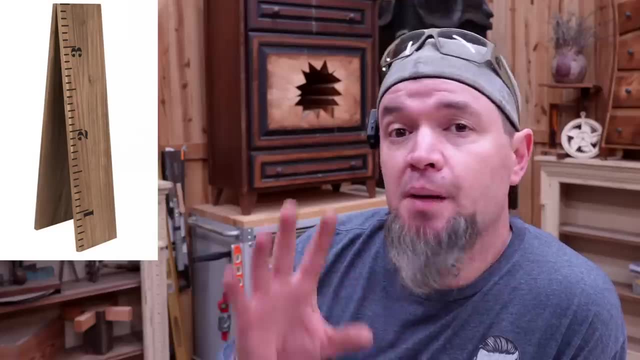 go with two of these. It would actually be cheaper if you just bought a 1x8x12 and you can pick those up for a little under $16.. So this is as simple as it looks. They've just cut their boards down into three foot sections, put a couple of hinges on the back, placed a removable wall. 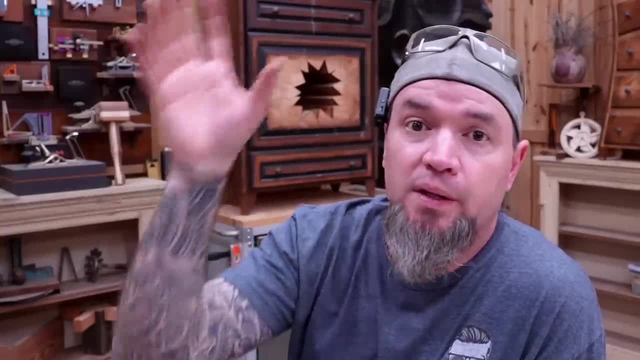 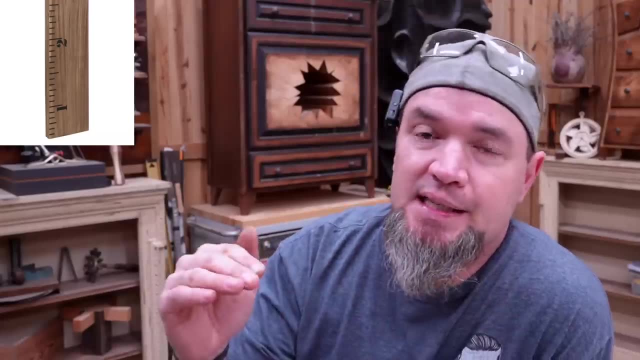 hanger on the back of the two boards while they were folded up, and then you could unfold it and place your second wall hanger on as the child grows. And if you're wondering why the one foot so close to the bottom, that's because they want you to hang this six inches from the ground. If 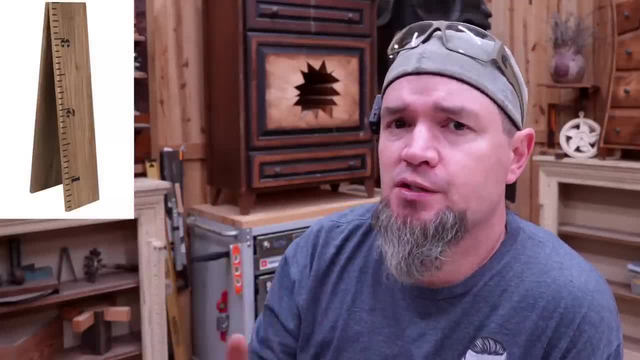 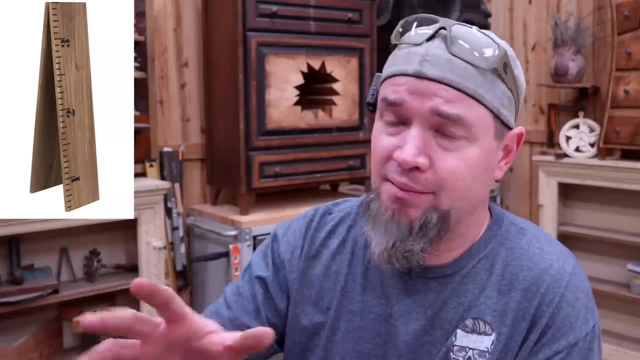 it were me, instead of hanging both of these boards together, I would just put the hinges on the back and have it to where it could be stored away and then added to it later. I just know how kids are and I know mine would be like smashing their brother's head in this thing, you know. opening. 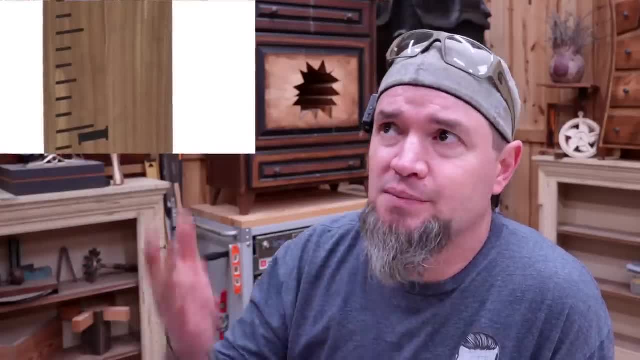 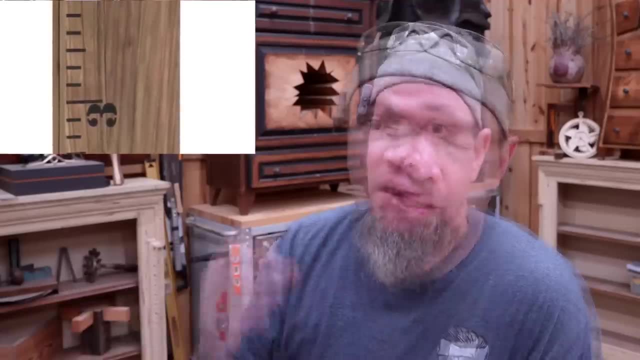 it up whatever. That's just how I would do it. As far as the lettering goes, stencils: You can actually pick up these number stencils pretty much anywhere, because these are the sizes that are intended for mailboxes- Easy to find Now. this would be a perfect project if you had a. 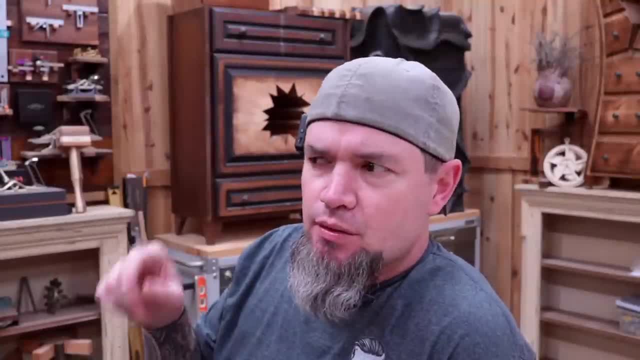 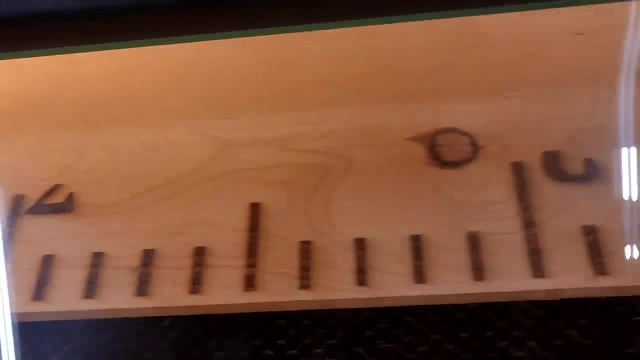 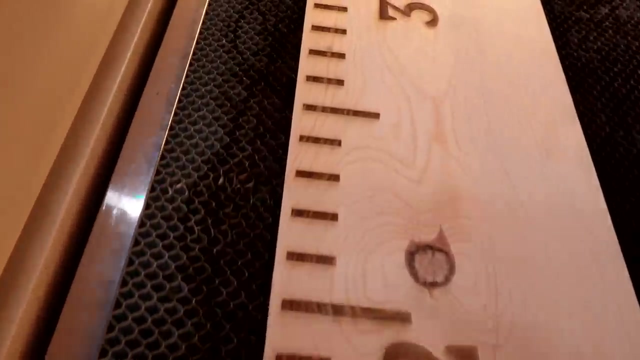 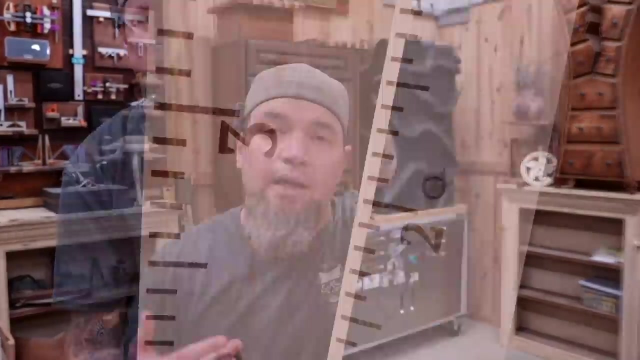 laser or a CNC, And I actually have an example in the Thunder Laser, so let's check that out Hot off the press, and this is what I'm talking about Now. if I was actually making this for a customer, the only other thing that I would 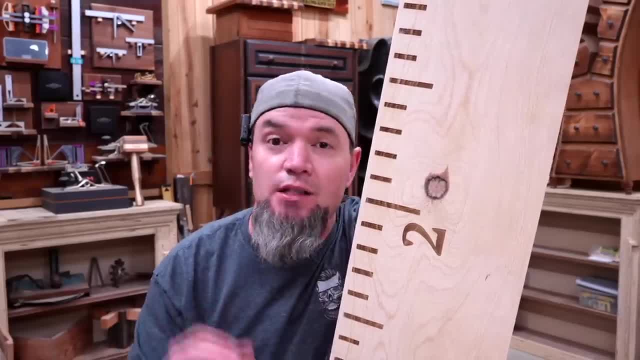 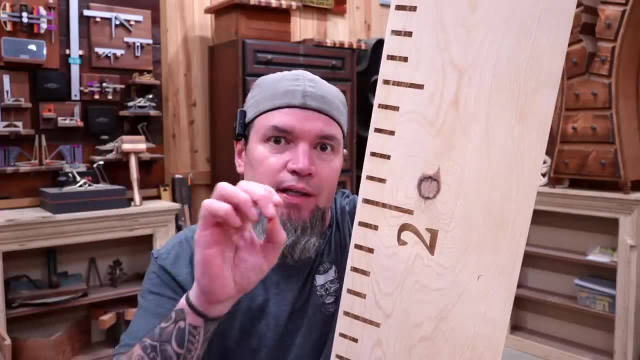 do is personalize this thing. Anything personalized will sell, And especially if you put grandkids names on this or even the family name Where, like the family tree, is growing Just little quirky stuff like that. People love it. It falls into one of 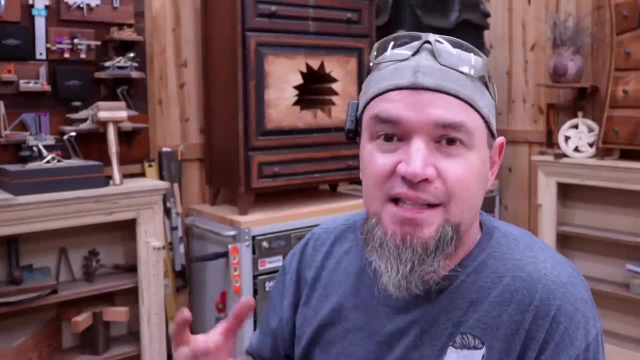 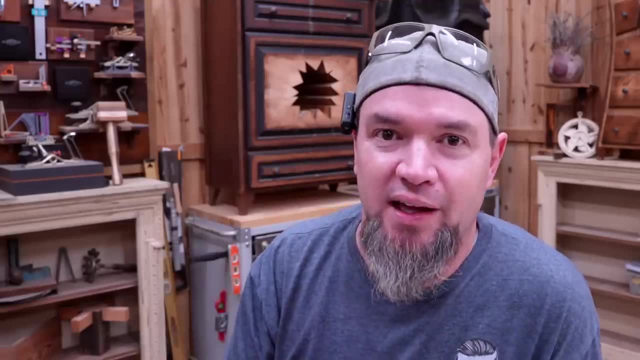 those categories that people will spend money on. A guaranteed sale is when it comes to spending money on someone's kids or grandkids, especially whenever they are young. It's kind of like the baby book thing: You know the firstborn. the baby book is like this thick and it has like the first. 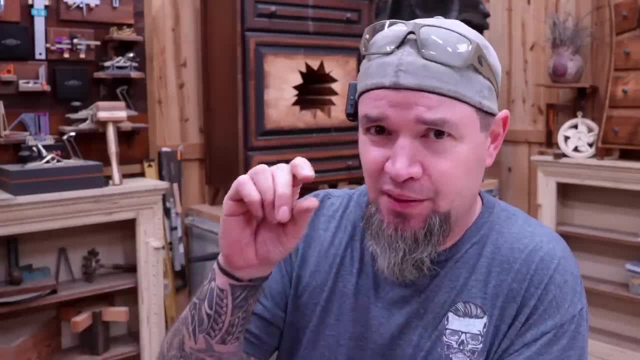 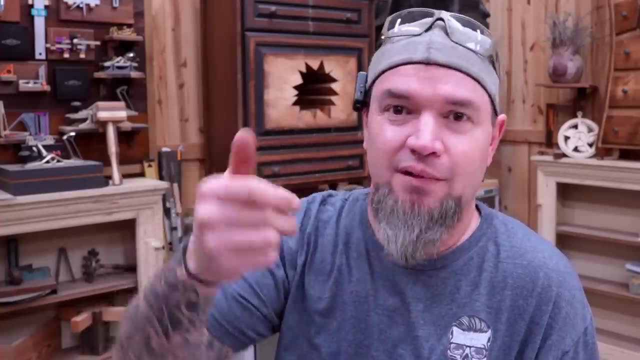 time that they pass gas in there. And then the second child: it's like a little bit thinner. And then, you know, it's like first birthday got this present. And the third child, you know, here's their book. So, all jokes aside, grandparents will buy this for their grandchildren. 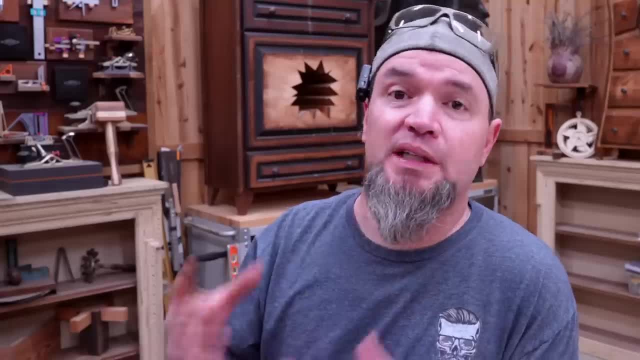 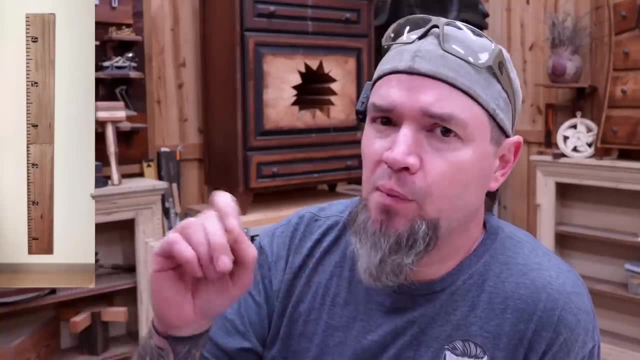 and grandparents are probably the one with the money. I would leave the wood, natural pine, because almost every ruler I've ever seen in my life has been made out of pine Plus. if you put any type of an actual finish on this, they won't be able to write on it unless it's with a permanent. 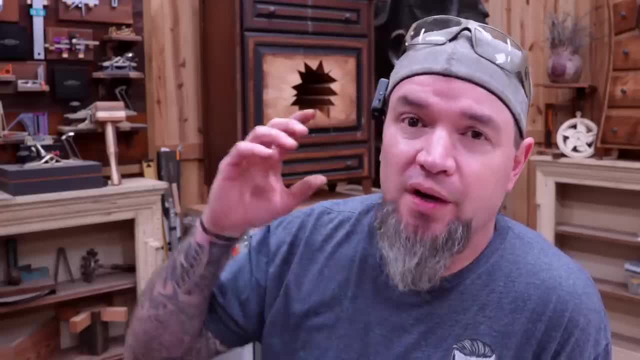 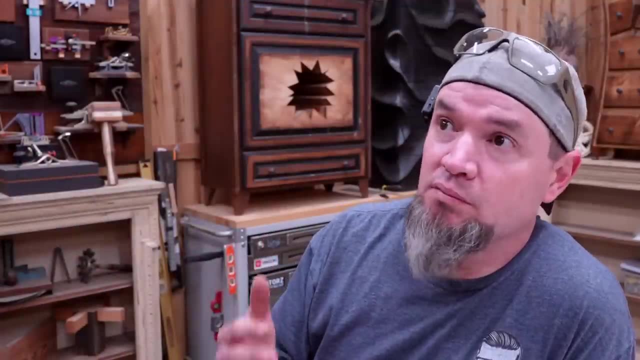 marker. So if you make these things up, they look nice. I don't think that you have any issues at all getting 50 bucks a piece for these. And this next one I personally thought was super cool because it's actually made out of reclaimed wood And it's this. 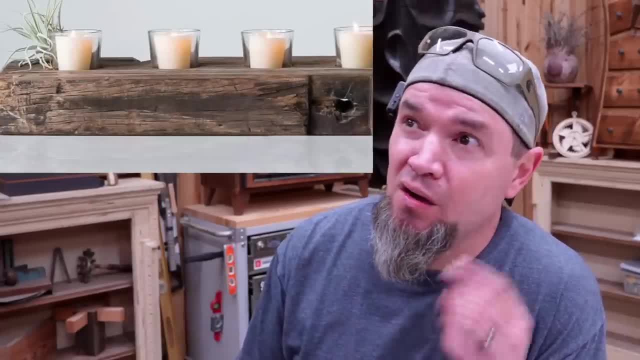 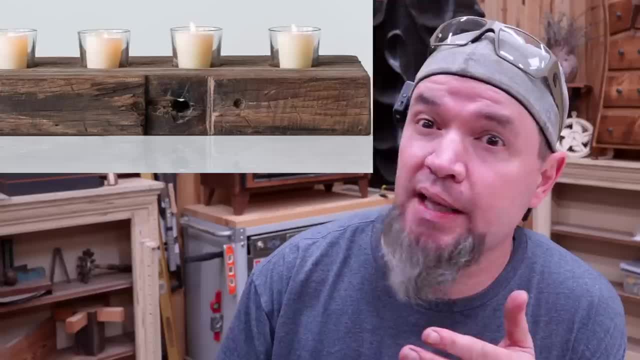 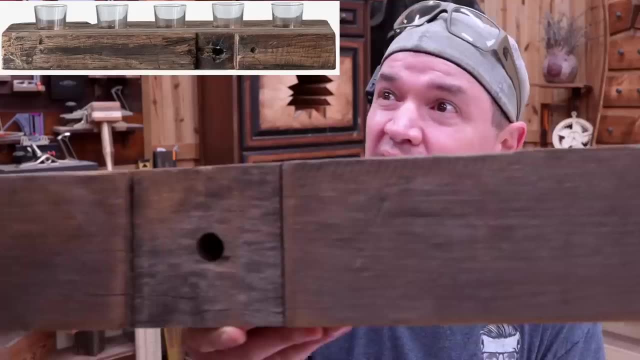 pick up for next to nothing. But honestly, I shouldn't even be showing you guys this thing, because for 90 bucks obviously they are the only place on earth that has access to material that looks anything close to this. I mean, look at that old bolt hole in the oak. 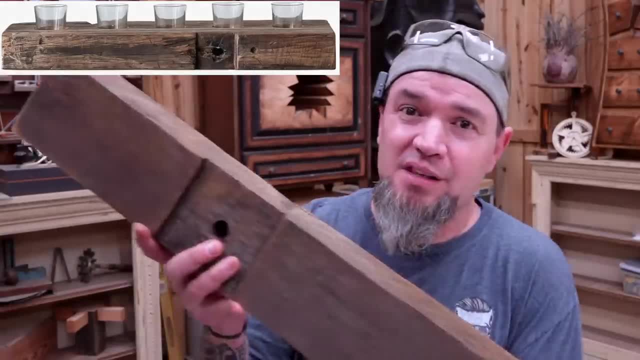 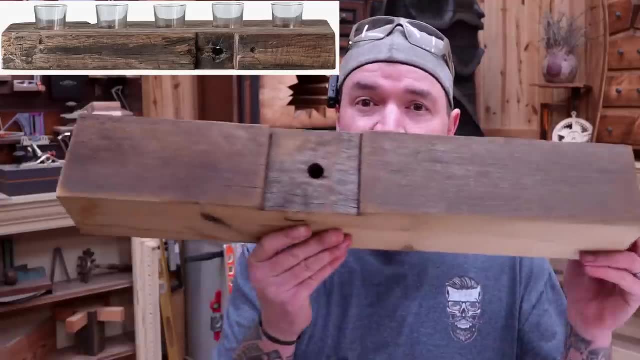 And no, I did not purchase this from them. I have a pile of this stuff laying around. It's reclaimed wood. When you are out and about, just look at, oh, lumber, that has potential. I mean, look at this thing, It's almost identical. 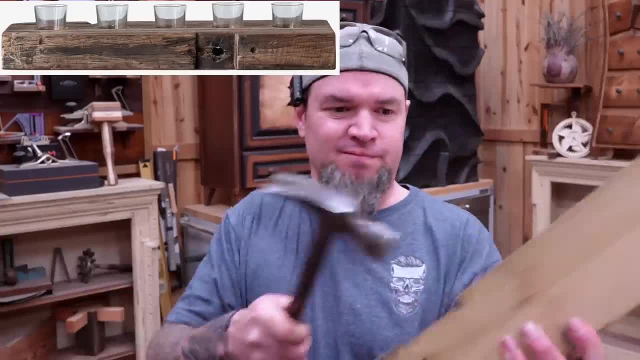 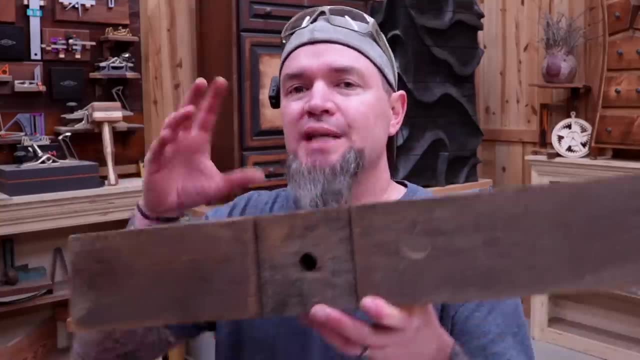 except theirs has a little dent close to that hole. Now it's identical and I can get 90 bucks for this. I bet if I hit it again I could probably get 100 bucks for it. All jokes aside, you can use any rustic piece of lumber that you have- old 4x4s, anything like that with this natural.